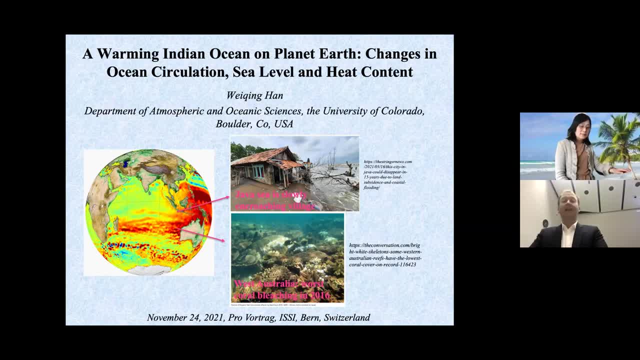 It has now recently changed, but before it was really difficult to come here. Therefore, we have this talk today in the form of a Zoom talk. We hope that next time, in March, then we will have our first normal talk again, But as you know, this is currently difficult, very difficult. 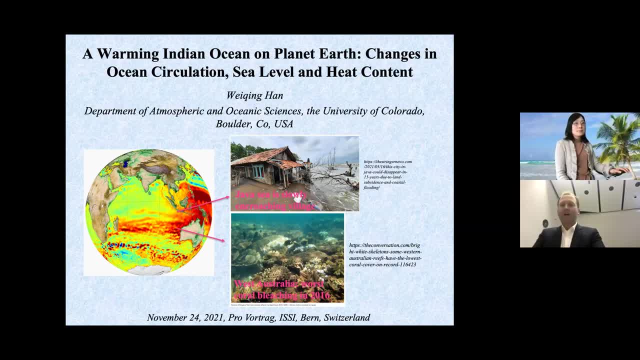 to predict what will be the further development of the pandemic, But in any case, I would like to introduce to you our speaker of today. So Wei-King Han obtained her bachelor degrees from Nanjing Institute of Meteorology. She then obtained her master's degree from the Chinese. 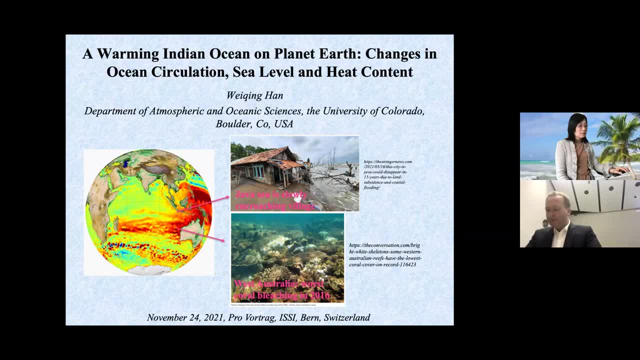 Academy of Sciences in Beijing. She then moved to the United States to obtain her PhD on physical oceanography from the Nova University in the United States. She then worked as a postdoctoral fellow at ATOC, so in Colorado, at the Department of Atmospheric. 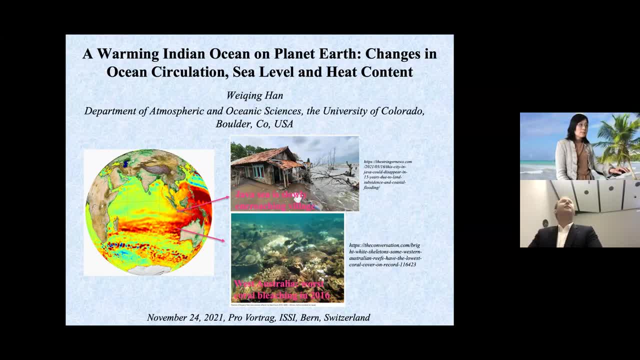 and Oceanic Sciences. She there became in 2002 assistant professor, then an associate professor And since 2016, she's a full professor at the Institute. She's a member of numerous different associations, like the American Association for the Advancement of Science, the American Geophysical Union, the Meteorological Society. 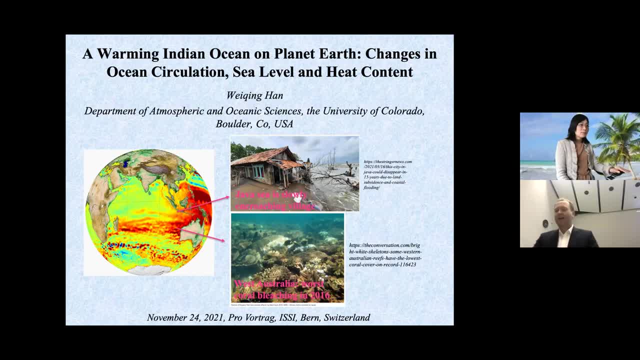 and the Oceanography Society, And she has had many honors, including a fellowship from the University of New York, the University of New York, the University of New York, the Excellence Cluster in the University of Hamburg, Germany, And most recently, in 2002, she was. 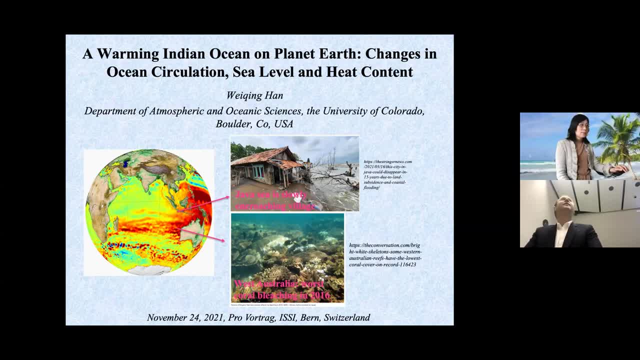 selected as Johannes Geis Fellow at EC, So we thank you very, very much for joining us today and giving this talk. Please, Wei-King, you have the floor. Thanks, Christoph, for the introduction. I'd also like to thank ISSI for providing the. 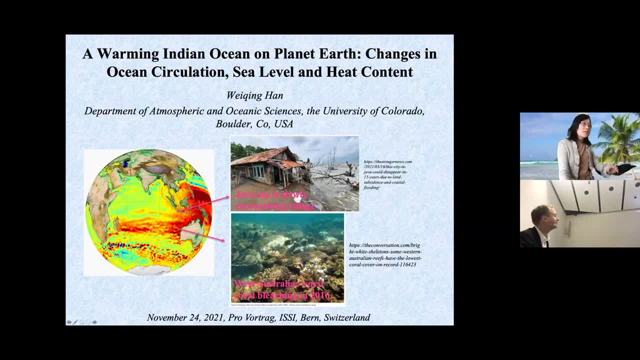 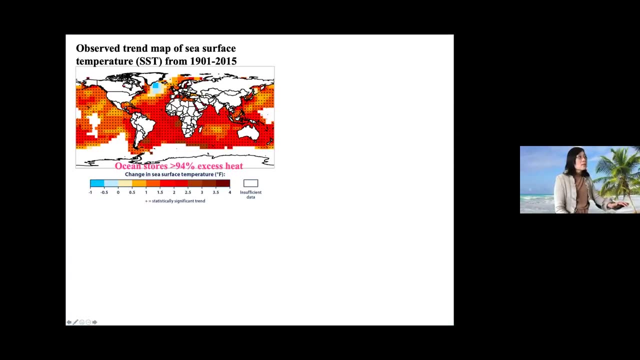 opportunity to give this talk, So today I'll share some of my research in the Indian Ocean, on the planet Earth and change the ocean circulation, sea level, heat content and their impact. So this is the trend for the observed sea surface temperature in 115 years, from 1901 to 2015.. 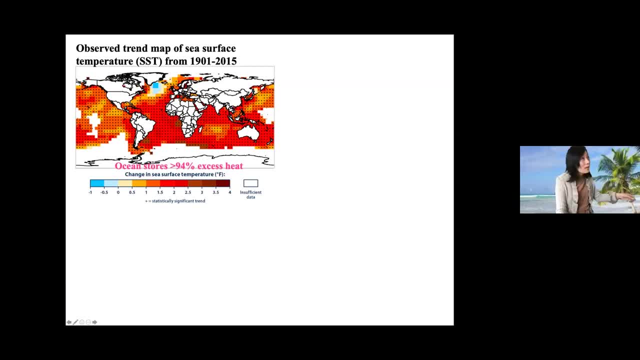 So the positive values here shows the warming trend, like the ocean is warming, and the negative values, like blue, shows cooling Due to the increased concentration of greenhouse gases in the Earth's atmosphere, which traps heat to the Earth's climate system. and this amount of heat- over 94%. 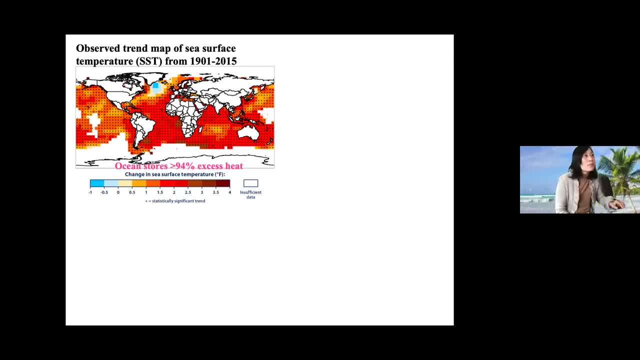 entered the ocean. Therefore the ocean has been warming. So the time series of this sea surface temperature anomalies, averaged in the global scale, also shows an increasing warming trend here based on this 30-year average from 1971 to 2000.. 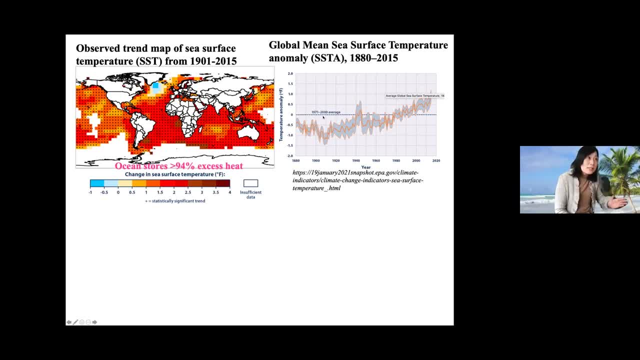 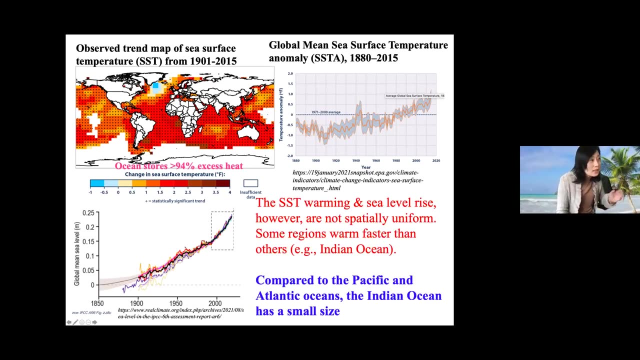 Due to this warming, due to thermal expansion and also melting land ice, the global sea level has been also increasing in the past century. So this warming and sea level rise, however, is not geographically uniform. As we can see from this SST sea surface temperature trend, there is stronger warming in the 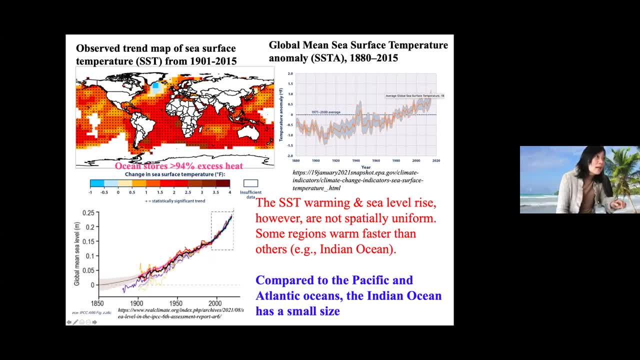 Chinese nation. It Russian Ocean unfortunately has relatively less human Canada and due to the smaller sea surface temperature in the world. What is απο gorgeous? The nation is smaller when compared to the group of defaults of the Chinese Grasslands. you will beget more based on the winemaking statistics that can be seen, as you can see here. 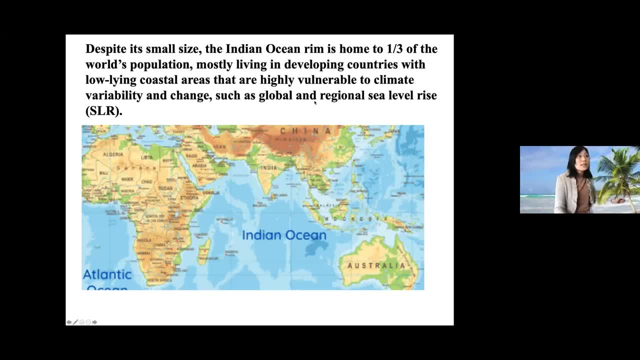 here To define the range of both. this engagement north to the east, that's OK. Therefore, since the behavior of lessenan area, we need to look at how the body heat, bekomens and Groundwater fulfill. So, like Baylenberg, the Indian Ocean has a пром практически solid body temperature in most parts of the Indian Ocean, Accompanied by a weak warming in the South Tropical Indian Ocean Basin. Compared to the vast basin size of the Pacific and Atlantic Ocean, the Indian Ocean is small. these by its small size, the Indian Ocean projekted to: 1: 1. 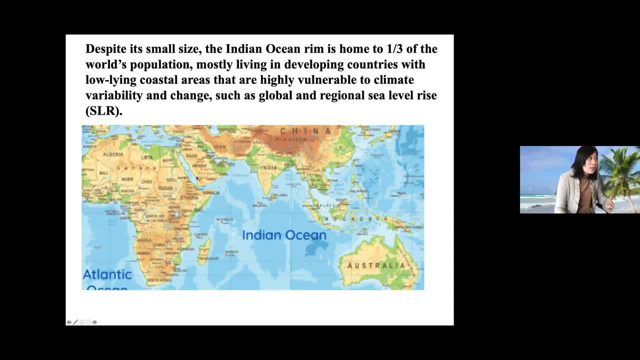 And, more importantly, most of them live in developing countries with low-lying coastal areas- here, as we can see, India, Bangladesh, Myanmar, here Indonesia, this side, Somalia and the African coast. So they are highly vulnerable to climate variability and climate change, such as global and regional. 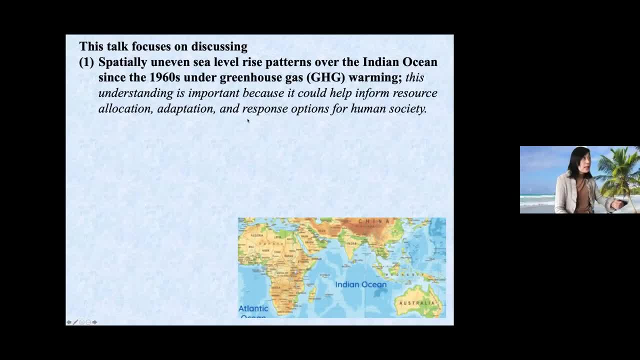 sea level rise. Okay, so here in this talk I first discussed the spatially uneven sea level rise patterns over the Indian Ocean since the 1960s under the greenhouse gas warming. So this understanding is important because it could help inform resource allocation. 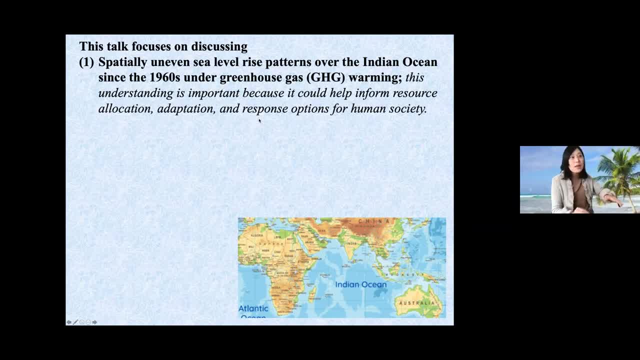 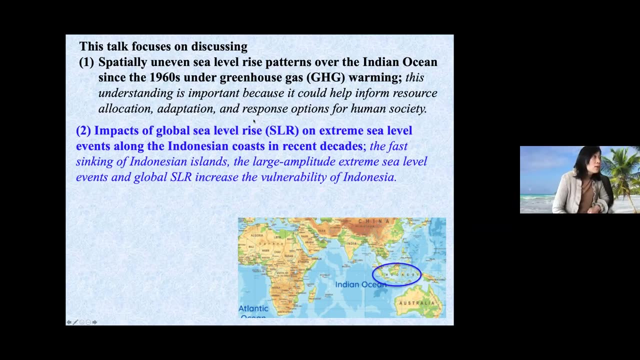 because if we have limited resources we can't allocate everywhere, but some very highly vulnerable places should be there. Okay, adaptation and response options for human society. Then I'll discuss a little bit the impact of this global sea level rise here on the. 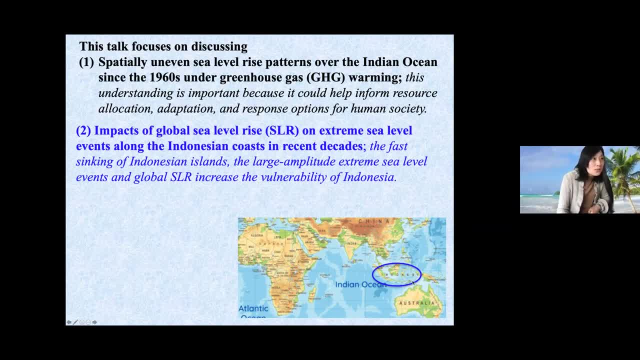 extreme sea level events along the Indonesian coast in recent decades And we know that the Indonesian islands have been subject to strong sinking and Jakarta, there The capital city, sinks the fastest among the cities in the world. plus, large and extreme sea level events and the global sea level rise increased the vulnerability of Indonesia. 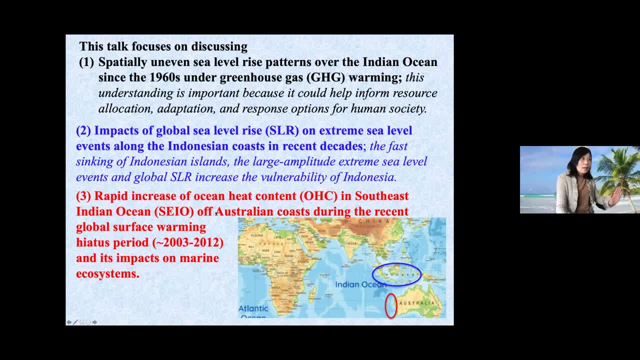 Lastly, I will discuss a little bit about this upward trend, like regional sea level trend, the interaction with the natural internal variability on the decadal timescale. So the rapid increase of ocean heat content In the Southeast Indian Ocean off the Australian coast here during the recent global surface. 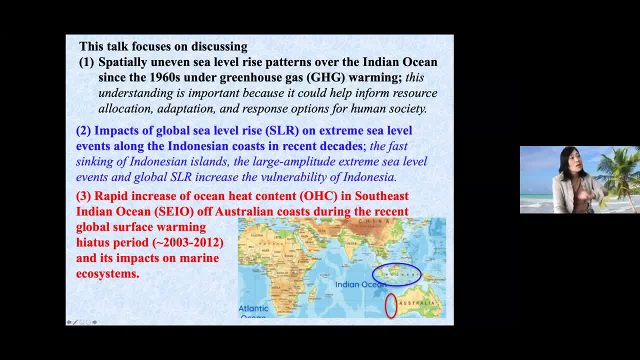 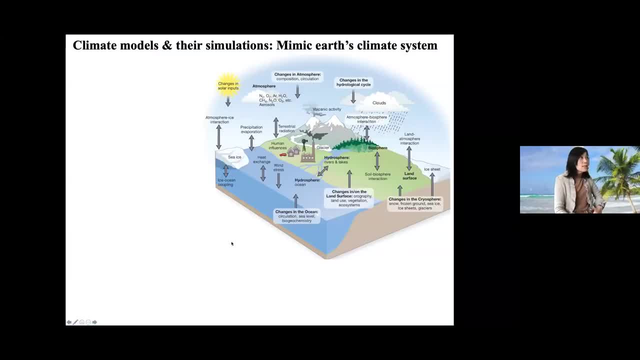 warming hiatus, like surface warming, almost stopped that period of time and this warming impact on the marine ecosystem. Okay, since this study, since here the rest of my talk will mention something about the modeling, like climate modeling and the ocean modeling here. 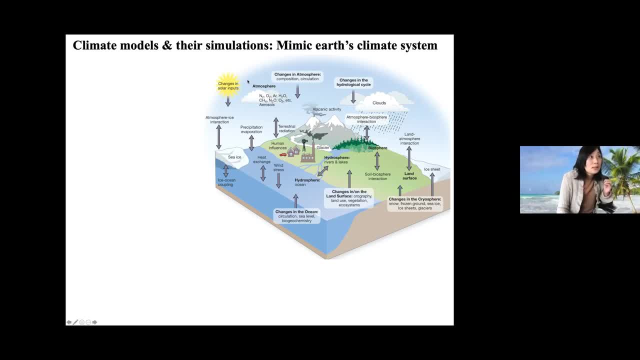 I'll briefly Introduce basic climate models. Okay, And here this is. this picture shows this real Earth's climate system. We have different component. We have atmosphere, We have heterosphere, lithosphere and biosphere. climate models actually mimic that's a realistic. 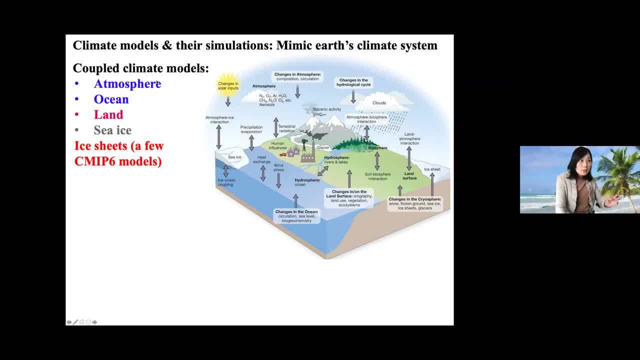 Earth's climate system. We have atmospheric model component, ocean model component, land surface model and the sea ice model. Some models also include this land ice, like ice sheet, Okay. And these different models? each of them are set of equations. 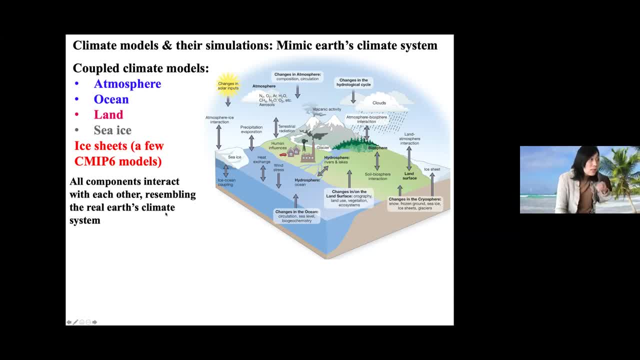 Okay, And they said all different components interact each other, which resembles a real Earth's climate system that with different component interact with each other. Okay, So using these model simulations, We can assess The impact of external forces such as greenhouse gas warming. 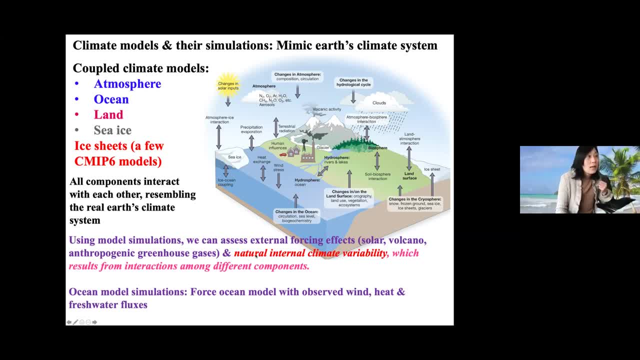 Okay, We will see part of those. Okay, And we distinguish them from natural internal climate variability. What does that mean? That means that even we don't have external forces such as the sun- see here, assume we fix the solar energy, come to the Earth's climate system, to a just mean climatological seasonal. 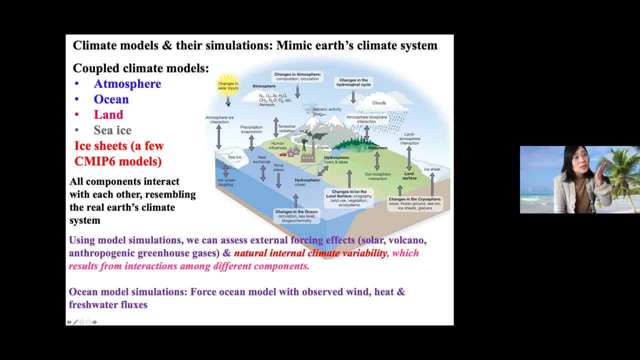 cycle And do not allow it Very from year to year And the longer time scale And also we do not have volcanoes and the no fixed, the constant greenhouse gas concentration, The interaction between all different components still produce variability and those variability, 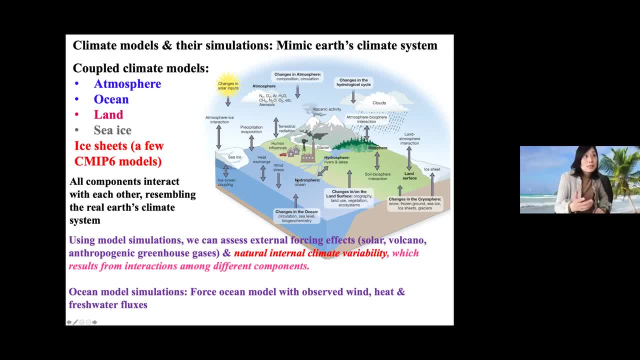 are natural internal climate variability. That's what we see like. this year is lining a year, right, That's part of, And so that's a negative phase of, And so that's natural internal climate variability different from the greenhouse gas forced variability. okay, and i will mention the ocean. 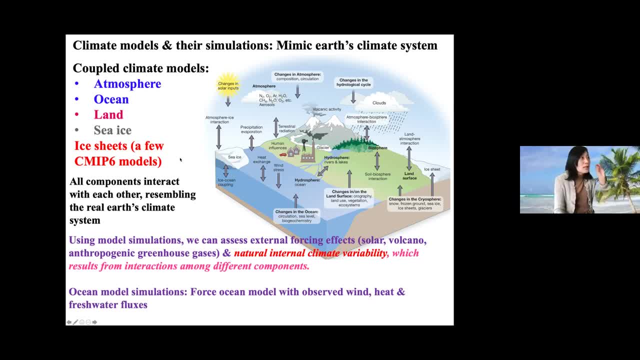 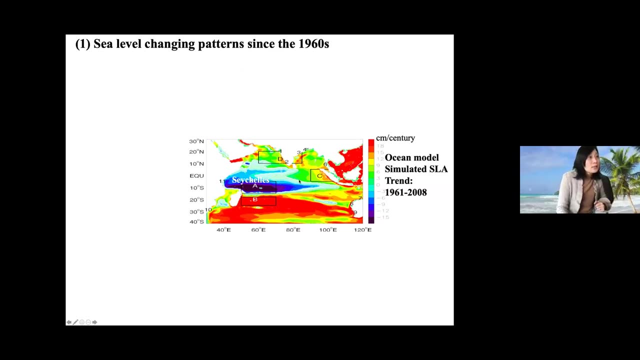 model simulation and this i just take the ocean model component and forced by the observed atmospheric wind and the fracture water flux and heat flux. okay, all right, first. so let's see the uneven sea level rise patterns. so this is the model ocean model simulated, the sea level anomaly. 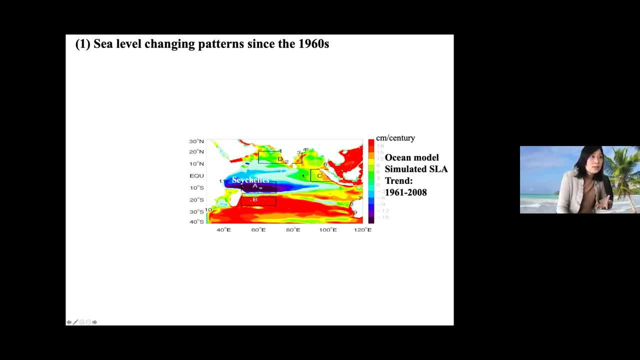 and for a 50-year trend. this is the trend, okay, from 1961 to 2008, close to 50 years, apparently- and we see a distinguished spatial pattern with the sea level rise along indian coast, bangladesh, myanmar coast and this indonesian coast, australia, madagascar, here, almost everywhere, except for this. 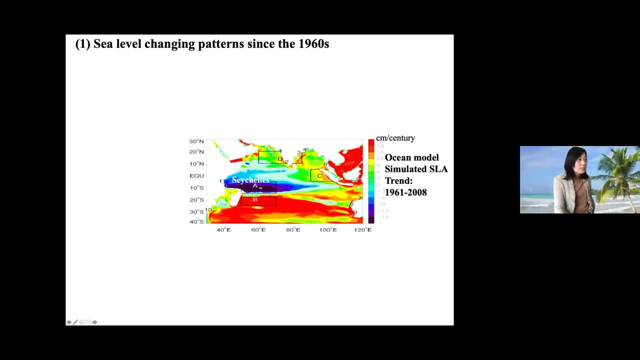 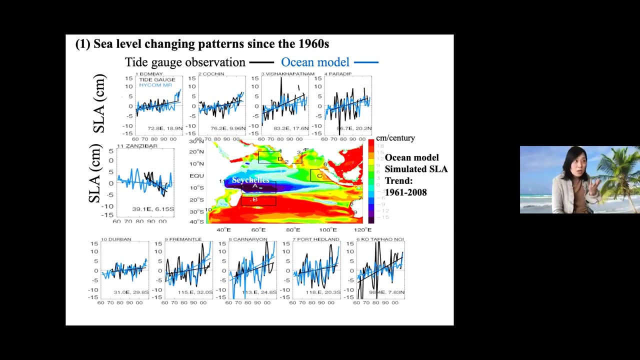 south west tropical union ocean seashores area. okay, and as we know here, here there is a sea level falling trend. okay, all right, so we know this is the model simulations. how about observations? we do not have such a long observations and for the basin wide scale, available everywhere. 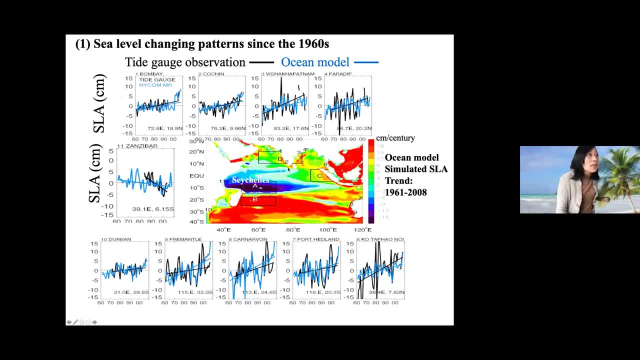 okay and based on that we i'll show here. but we have tight gauge observations along the coastal areas and the island region. here i choose this tide gauge data that has the links 20 years and longer. so here around here the black line shows time series of the tide gauge observations at each of the 10. 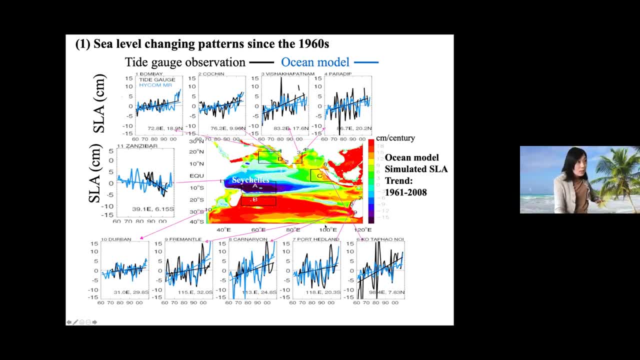 locations here around the indian ocean coast, as you can see, and this blue line shows the model simulated sea level. anomaly, apparently, both the tide gauge observed and the model simulated sea level shows a rising trend almost at everywhere along this indian ocean coast. okay, everywhere, except for zanzibar here. 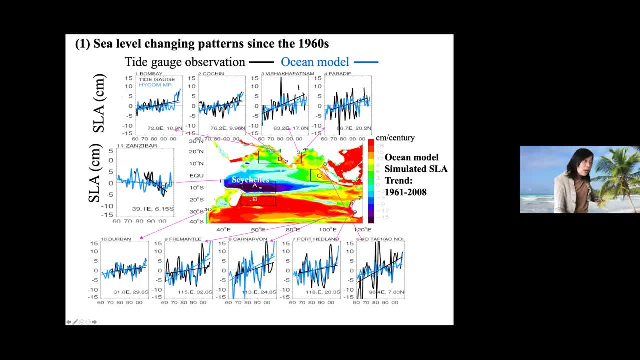 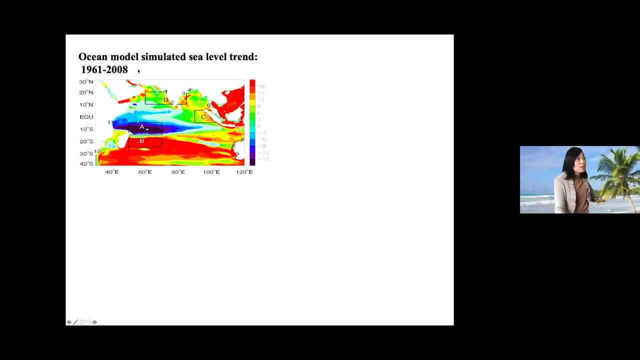 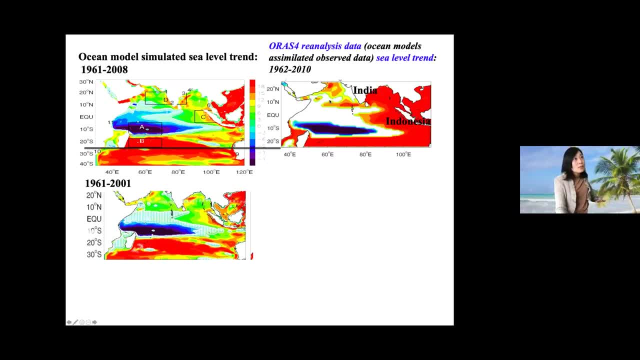 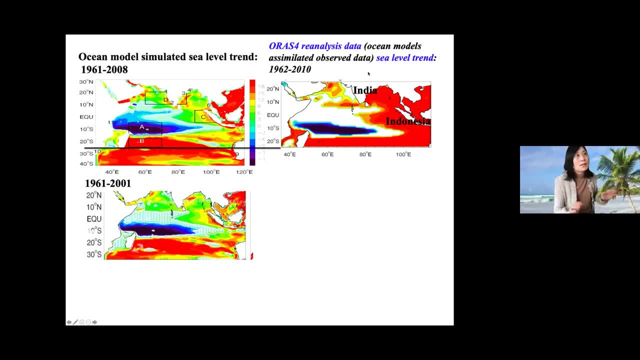 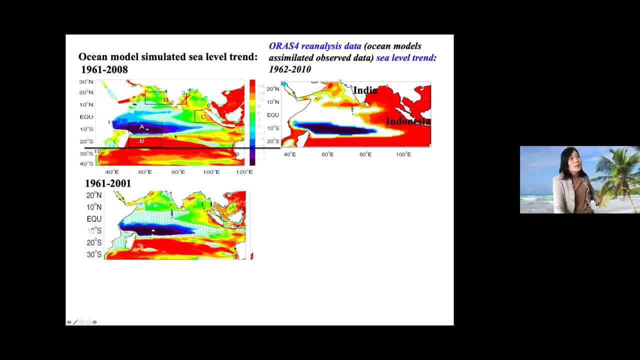 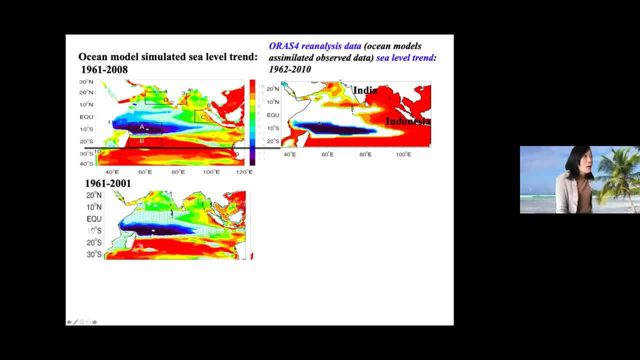 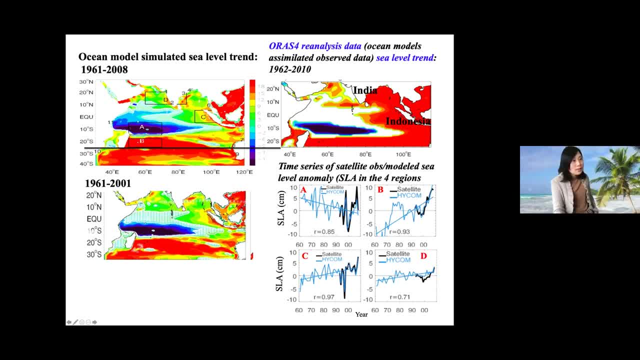 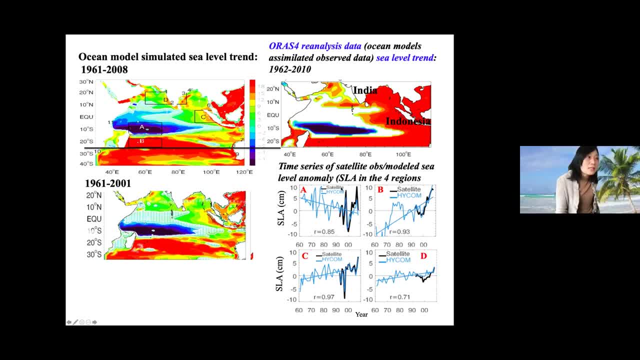 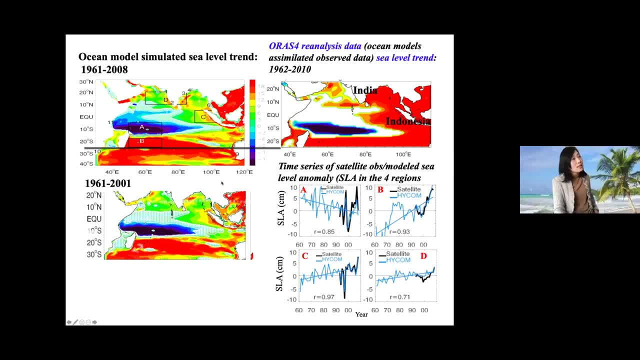 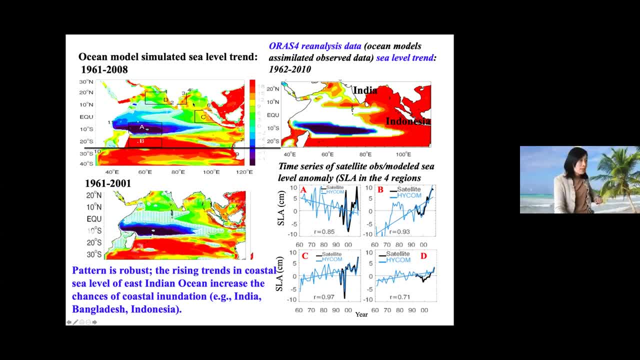 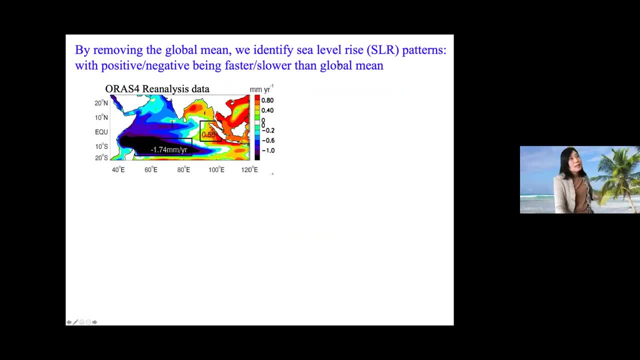 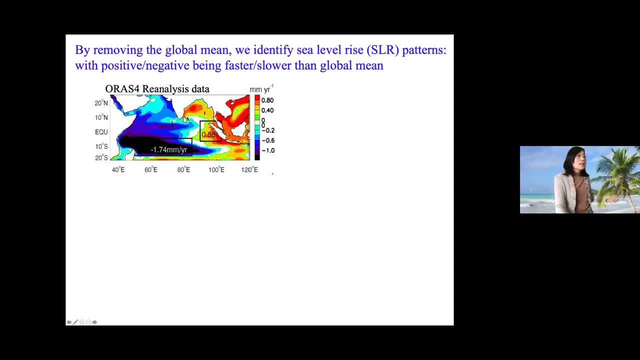 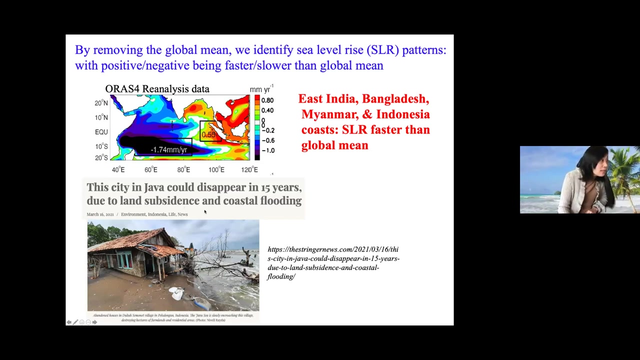 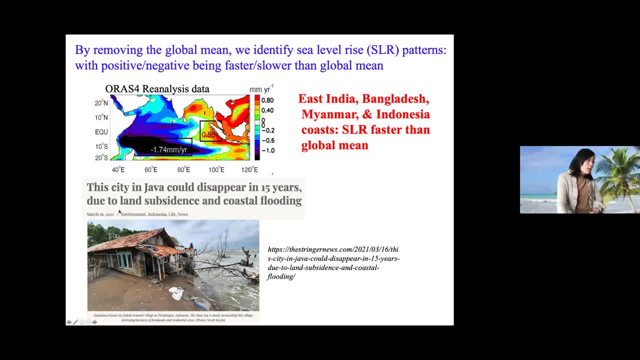 We're seeing that this is from March 16, 2021, this year. okay, This is news. And the city in Java, which is right here, the city in Java could disappear in 15 years due to land subsidence and the coastal flooding. So, and here we show that there is a multi-pecadal trend of a sea level. 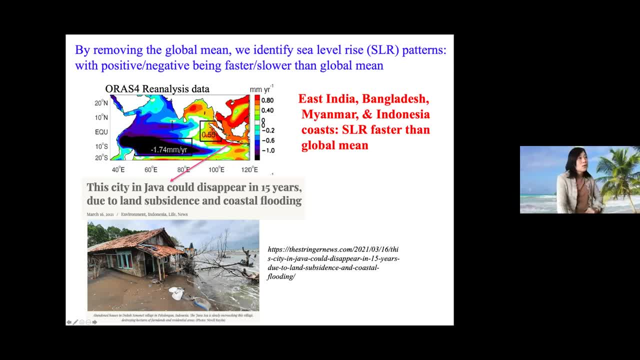 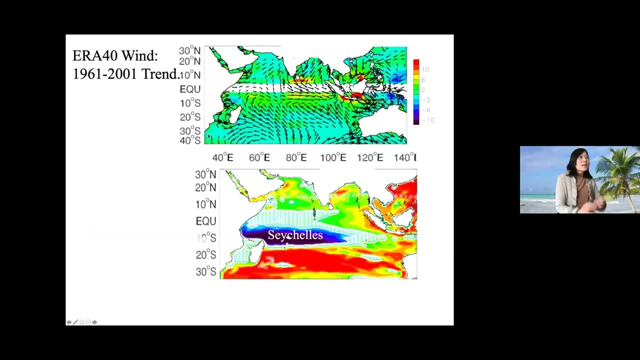 also rising here, showing that the sea level rises much faster than the global mean along this Indonesian coast. All right to understand why there is such a pattern in the multi-pecadal sea level trend. so here we did a model experiment. but here it only shows this surface wind pattern. 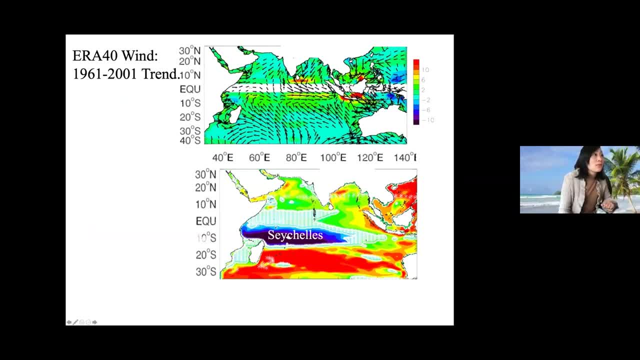 and those arrows here okay, show the surface wind trend. okay, for the same period of time as this sea level trend here. So in the ocean. briefly, I won't go into details, but one thing I wish to introduce is that for what we call the westerly wind, the wind blow from west to the east. 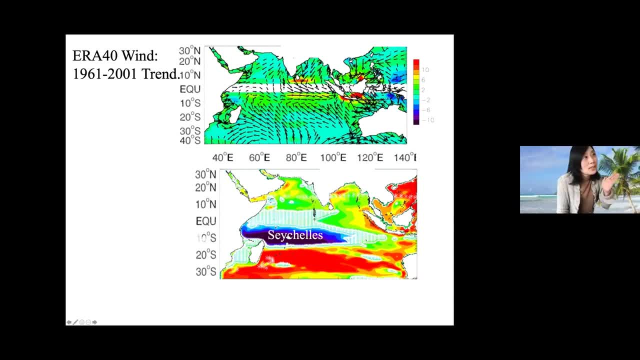 in the ocean. it causes not only eastward current along the equator, but also this ocean mass, like surface water, converges to the equator like this, because when the wind blows from west to east, because the earth's rotation and the 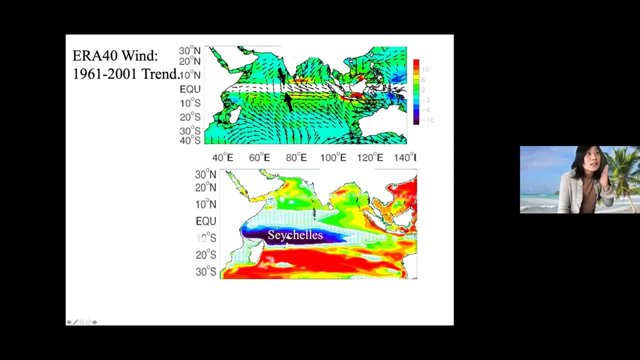 cryolite force causes it to be 90 degrees to the right, okay, and in the northern hemisphere, and then 90 degrees to the north, degree to the left of the blowing the wind direction blowing here, okay, and in southern 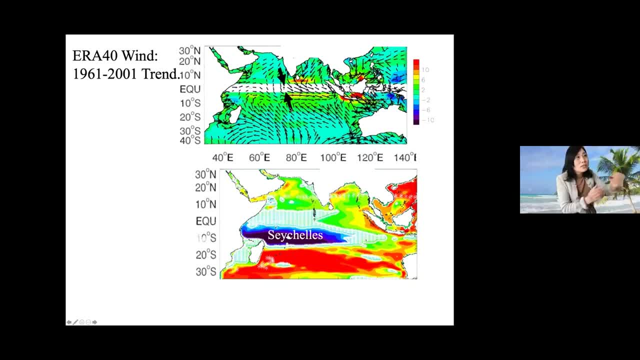 hemisphere. Therefore the surface warm water converge to the equator and then the west wind- the wind blow from west to east- also produce eastward current. okay, that carries warm water to the eastern boundary, and when they impinge on the eastern boundary they 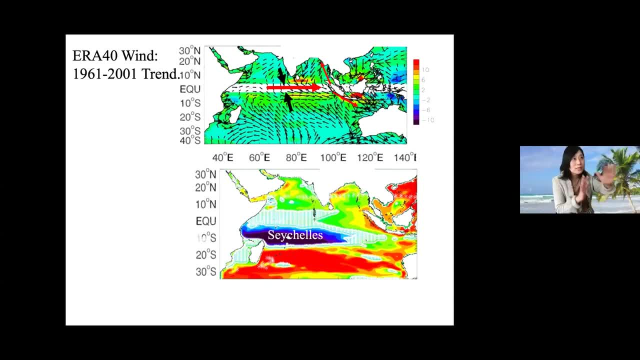 okay, transient signal is coastal carbon waves, but here we only we just want to. I just want to say that when the mass reach the distant boundary, it also flow poleward along the coast. Therefore, as we can see here, we produce the high you accumulate. 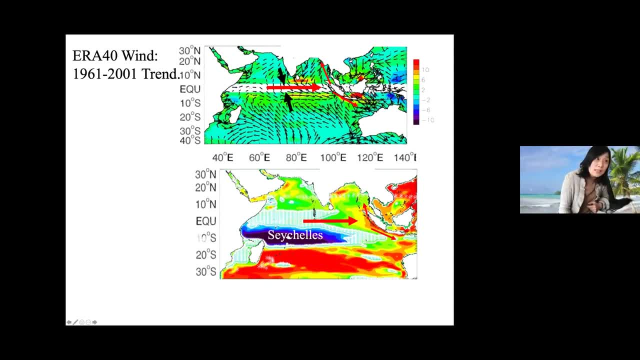 the water, warm water, which is high sea level here and also spread poleward along the coastal area, So you can see coherent sea level. Yeah, Okay, increase along the indonesian coast. okay, all right. so for the open ocean here. why does here all of a? 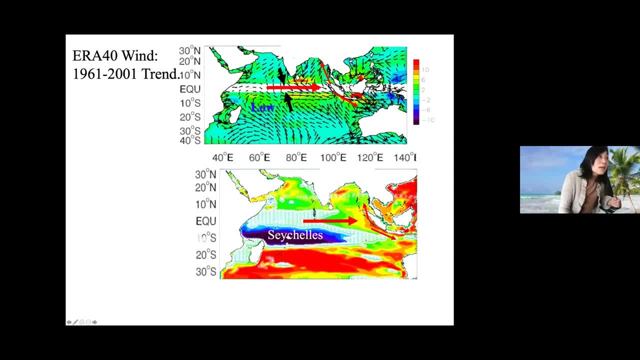 sudden get a blue like a sea level. four: look at the wind pattern, clockwise, if you, if we think about this southern hemisphere and acumen, we call it acumen transport, which is oceans, the seawater surface, warm water transport is in 90 degrees to the left, in the, to the wind, the wind below. 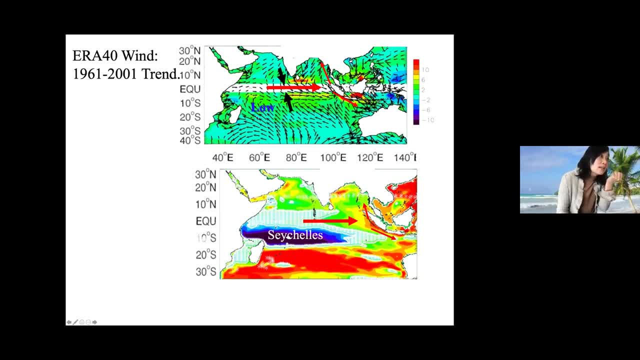 this way. so 90 degrees to the left is here southwest and here 90 degrees to the west is westward, here is northward. okay, so this means surface mass diverge from this area when you have clockwise when pattern, so the warm water is removed, cold water comes up from the sub surface. 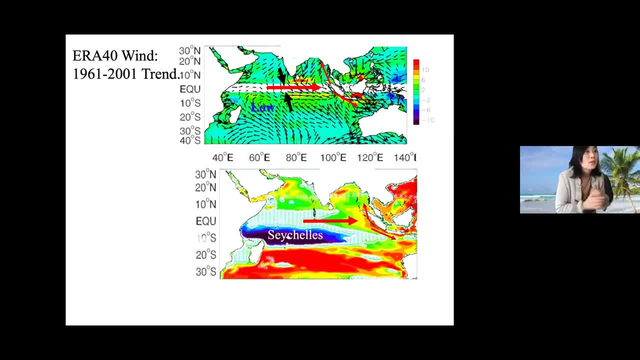 and above the bottom of the ocean you can see, see the interstices come right here. that's the allocated around the ocean. so the surronding surface, isamas water, is still's cookies, особенно in the development of the ocean. left is one of theppers of the downwardulf. now, if you look, 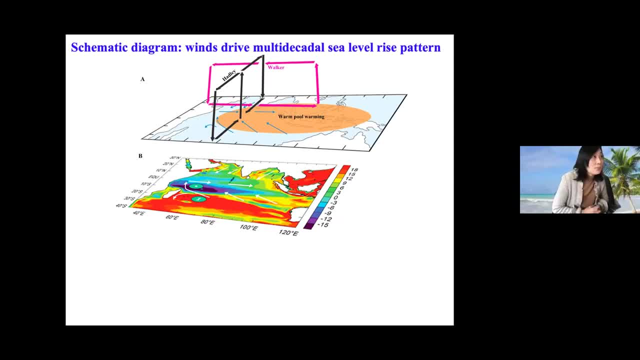 at the across the ocean longBeach portion that the urban longer televisionaat Consonant enough time to move in this direction is gone up. you don't have any more signal again. it is only left and right already. right circulation we call the work circulation. If we perform this, meridional mean like a 25 degree. 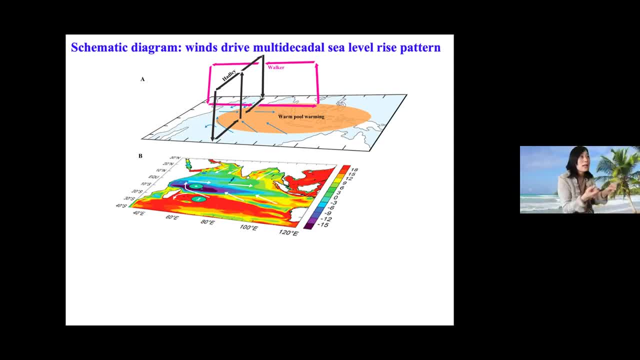 north, 25 degree north, let's perform the mean so we get an east-west circulation pattern. So with the warm air go up over this warm surface ocean, warm air goes up in the East Indian Ocean and the upper level go west and sink down to a relatively cooler sea surface temperature area. 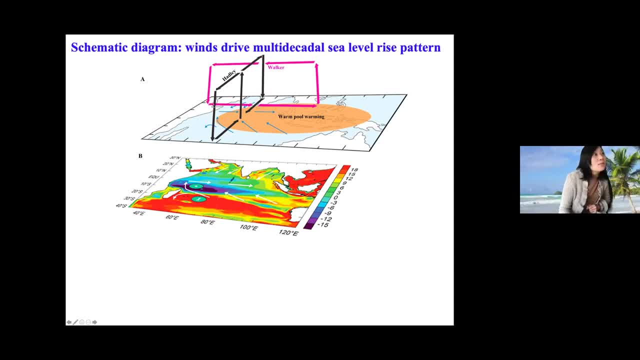 and then flow eastward at the surface, Therefore. so west the wind, the westerly wind that blows from west to the east at the surface, okay, is the lower branch of this enhanced work circulation, and this we call this wind, the surface. this wind produces this clockwise wind. 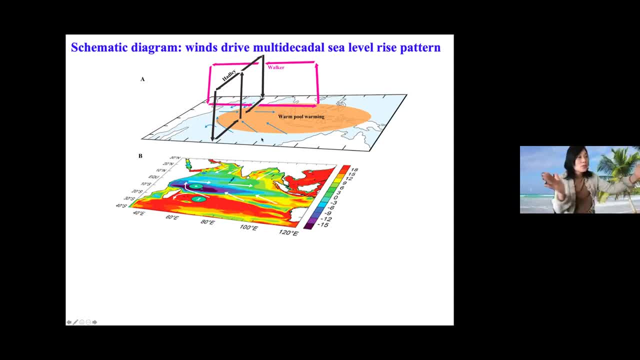 pattern: northern hemisphere, southward. If we perform the Zonglong mean you obtain this meridional atmospheric circulation and this northward wind in the southern hemisphere. southward wind in the northern hemisphere, like the blue arrow, is the surface branch of this hard-line circulation. 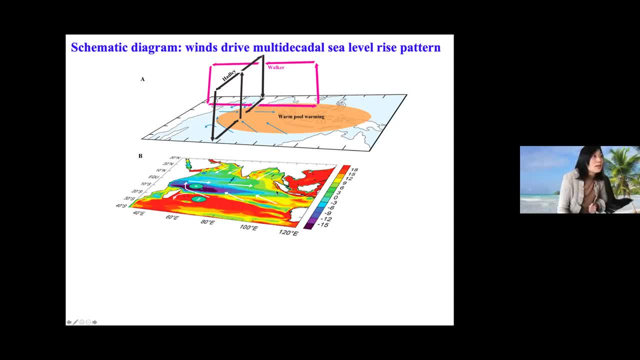 Therefore, this intensified surface-bound pattern that drives this unique or distinct spatial pattern of sea level represents intensified work and hard-line circulations over the Indian Ocean region. Okay, so here that's what I just said: surface wind, part of this intensified atmospheric circulation. 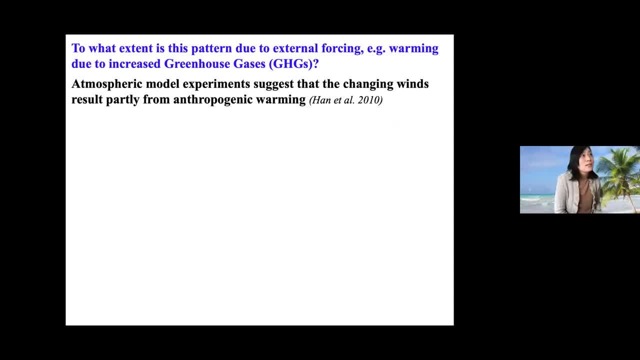 All right. so to what extent is this pattern of this surface wind result from anthropogenic greenhouse gas warming? And actually, in the early work, my co-authors and I we did a series of atmospheric model experiments and forced by different surface sea surface temperature, showing that this surface wind pattern results partly from anthropogenic warming. 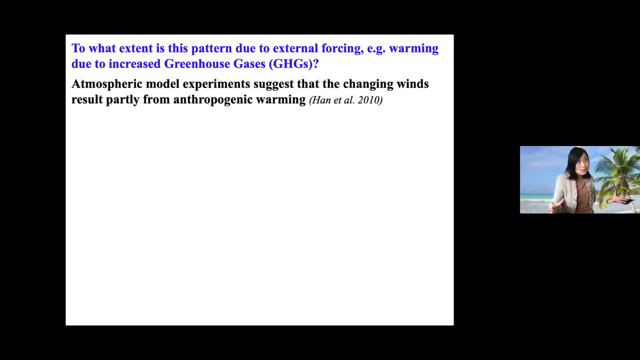 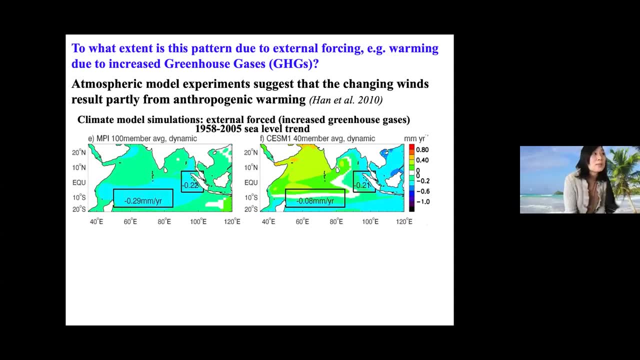 maybe other part from natural, as we mentioned earlier, internal climate variability. Then can the current climate models simulate this greenhouse gas warming? As I mentioned earlier, we can use these climate models, okay, to assess climate models, Okay, To assess this greenhouse gas warming. 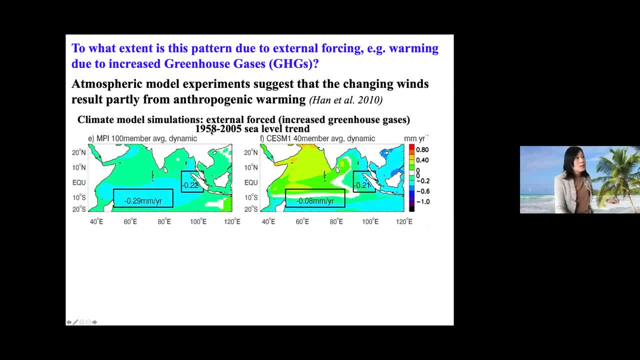 So this is a sea level trend from 1958 to 2005.. That's from a 100-member ensemble average. What does this mean? This means purely represent multi-equator trend forced primarily by greenhouse gas warming. Of course there's the volcano stuff, but for over 50-year trend, primarily represent greenhouse gas warming. 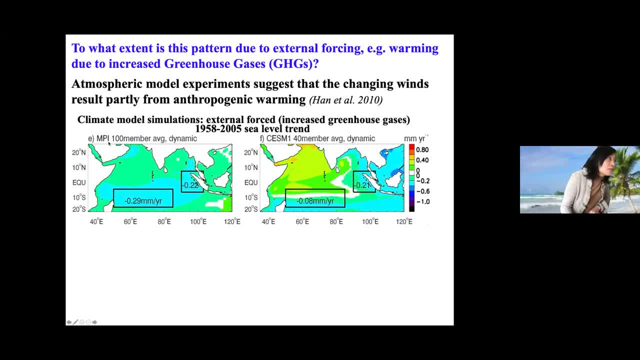 Okay, This is from Max Planck Institute of Meteorology, A 100-member ensemble average, And this one from the National Center for Atmospheric Research here in the US 40-member ensemble. So these represent sea level spatial patterns forced by greenhouse gas warming. 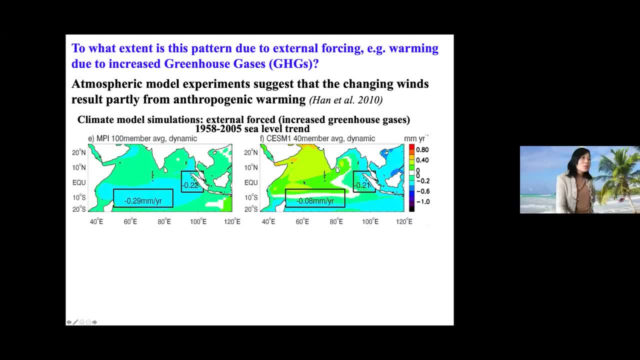 Unfortunately, although both produce some sort of spatial pattern, but they do not agree well. But MPI model shows better agreement with the observed assimilated pattern I showed earlier, With sea level fall over seashells and a relatively low sea level rise or slower sea level fall or sea level rise in other parts. 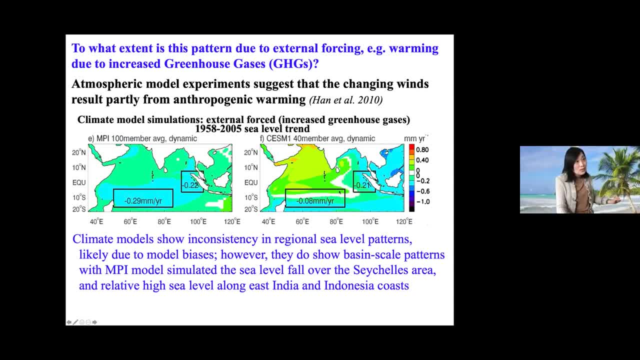 But the NCAR-CESM has much larger bias. Okay, So we also analyzed other, like the recent new SEMI-5, like IPCC, the sixth assessment climate model result, But they do not agree, Although our statement is: you know, it's not 100-member ensemble. 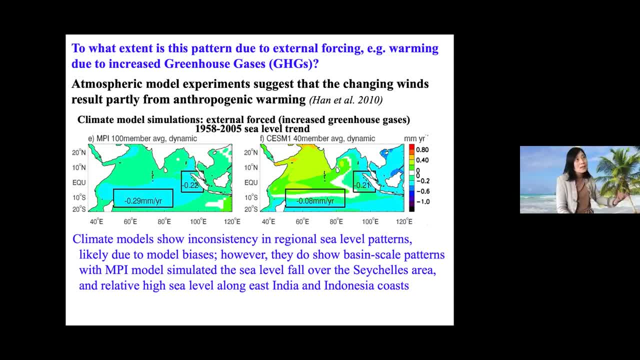 So our state-of-the-art climate models can simulate global greenhouse gas warming on global scale And also the global sea level rise due to the thermal expansion caused by the insupergenic warming, But on regional scale they do not agree. 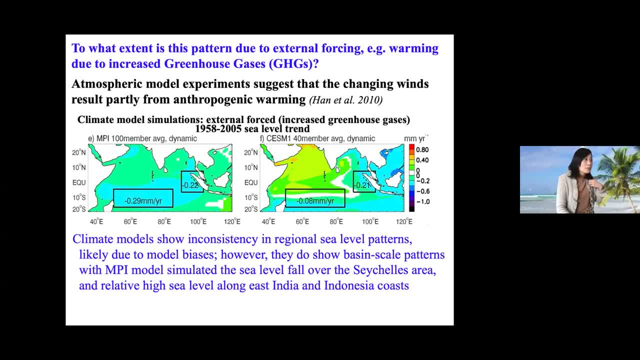 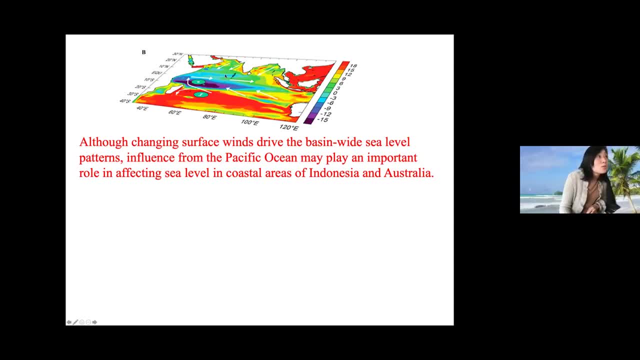 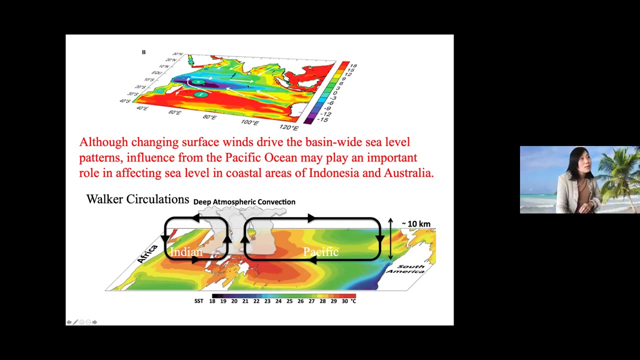 That's you need more work to improve the model. Okay, So, although the basin-wide surface went, it's the major driver for this distinction. Okay So, we have this distinct spatial pattern throughout the whole Indian Ocean basin And we know that this- Indonesia and Australia- sits right between the East Indian Ocean and the Western Pacific Ocean. 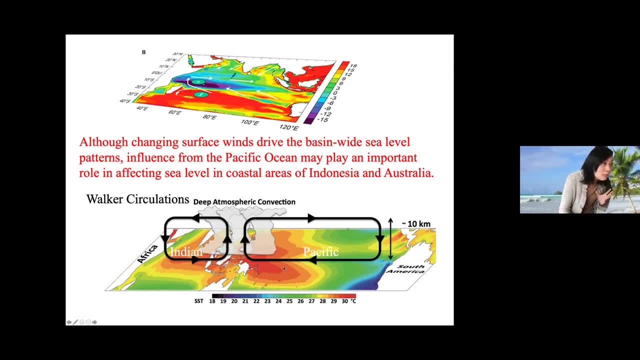 So here This is the mean pattern of sea surface temperature as you see the color And the white here show cloud like atmosphere convection ratio And the blue here shows the water circulation I mentioned earlier. So this surface here branch from the east to west. we call it easterly trade wind over the Pacific Ocean. 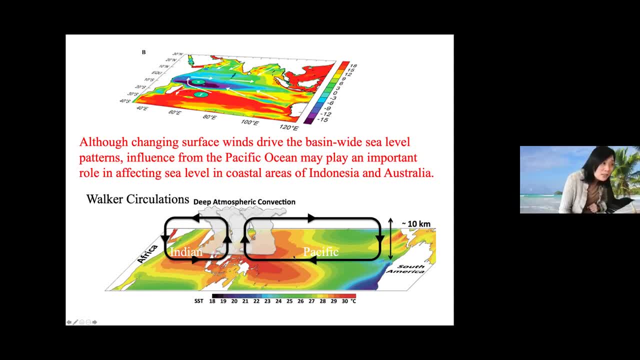 Okay, So when we have enhanced easterly trade wind, it will power up warm water to the Western Pacific And therefore it will increase this warm water that flow from the Western Pacific to the Indian Ocean. We call this part the Indonesian through flow. 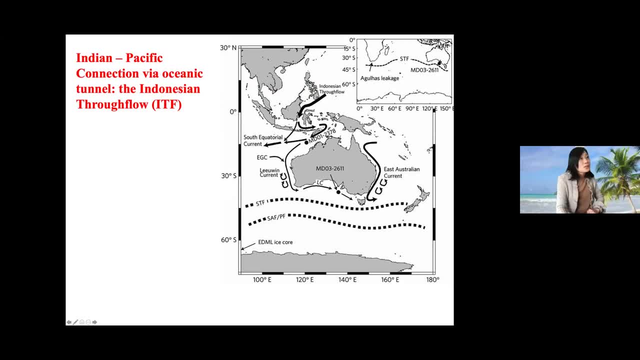 Okay, So this figure further shows a more clear picture of the Indonesian through flow. On average, the warmer and fresher water flows through here, from the Western Pacific into the Indian Ocean, through the Indonesian archipelago here, And also strongly affect West Australian coast and the Indonesian coast. 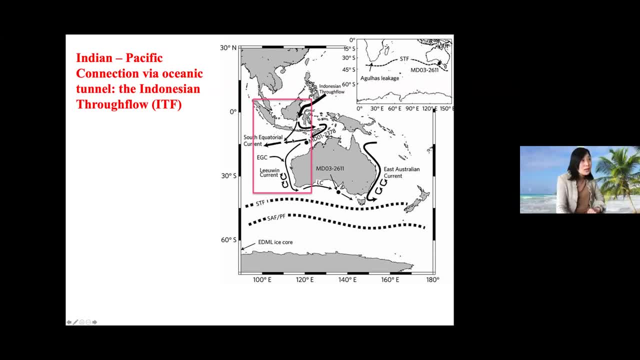 So the rest of the talk, we will focus on this. Okay, So the last part of this talk will focus on the two areas: This area very vulnerable, and the lack of resources to combat climate change. But meanwhile, the land is sinking fast. 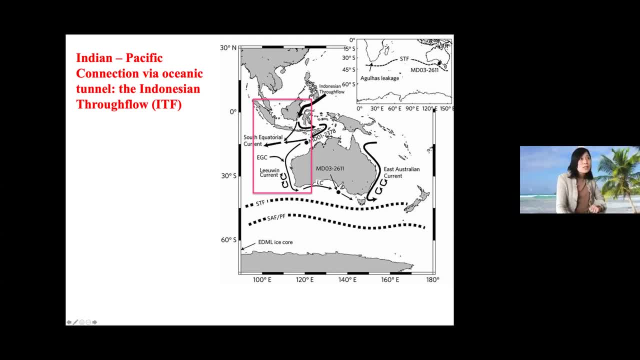 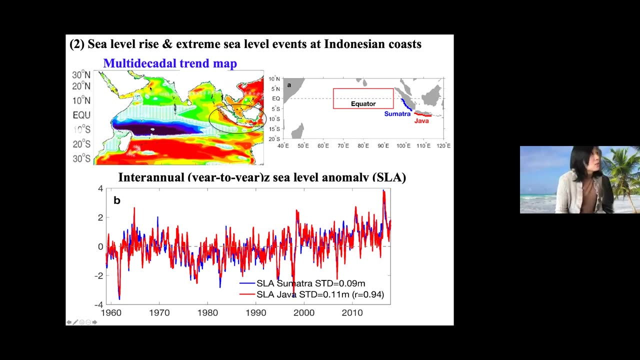 Okay. On the other hand, three sea level events really have large amplitude in this area And we also discussed here West Australian coast, Okay. So here I bring up this trend map again here along the Indonesian coast. here, all right, we see coherent locals- this is Sumatra and this is Java- and coherent sea level rising trend on multi-decadal time scale. okay, here and here sea level rise faster, is faster than the global average, okay. 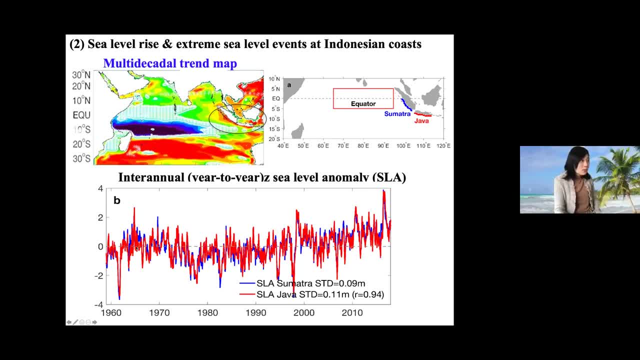 All right. so next I'll look at this time series of sea level anomaly and averaged over southern Sumatra coast, that's blue. and averaged along the Java coast, that's red. all right, and as we can see clearly, this is the upward trend. even we can visually identify here we have a sea level rising trend. agree with this sea level trend pattern? 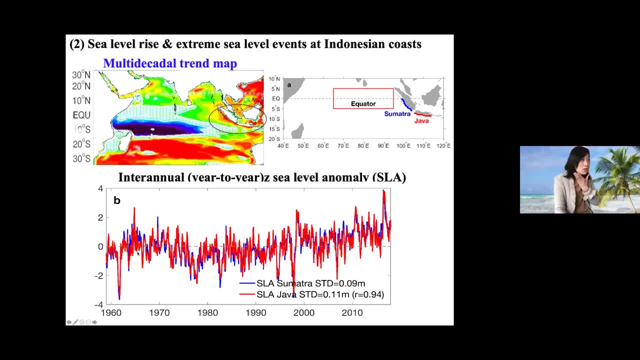 okay, As we discussed earlier, not only the two Sumatra and Java coast has coherent upward rising trend, but also have coherent sea level variability and these are based on monthly mean. okay, we remove the climatological seasonal cycle. this is just change from year to year, from decade to decade, as you can see these anomalies along these two areas also highly coherent, okay. 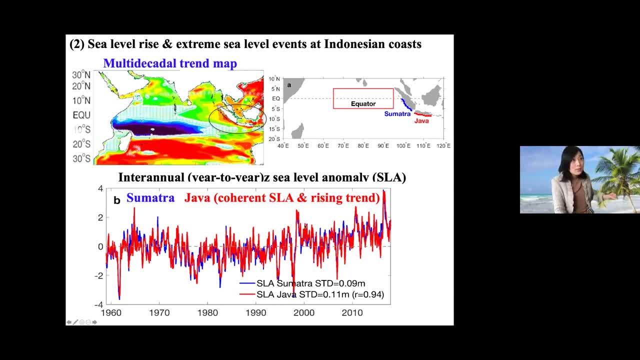 We'll discuss later why this is the case. Therefore, and next we'll primarily discuss the Java coast, because it has slightly larger variability, magnitude in sea level and here, as we can see, the sea level extreme- okay, high sea level, even in 2016, and reached the amplitude 0.45 meters on monthly mean time scale: half meter. that's huge. that's very, very high okay. 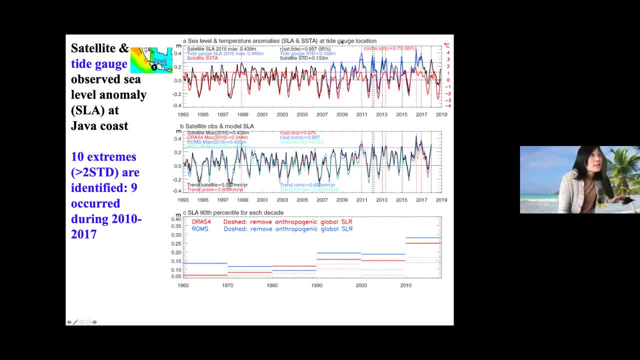 All right to detect, to detect this extreme sea level event and to define extreme sea level event, we use a sea level, we use a satellite. observed sea surface height observations, which is the black line, okay, and the tide gauge observations, which is the blue line, here at Java coast tide gauge station, this location at Java coast. 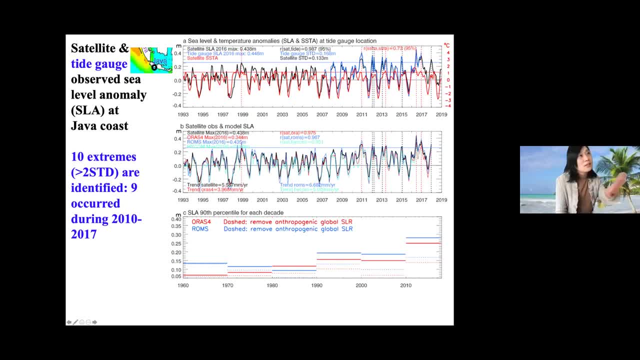 Okay. The red line shows sea surface temperature, but here let's forget about this one, we won't discuss that, let's focus only on this black line. the satellite observations near okay, the nearest location at to this tide gauge, okay area, which is about 18 kilometers southeast of this tide gauge location. 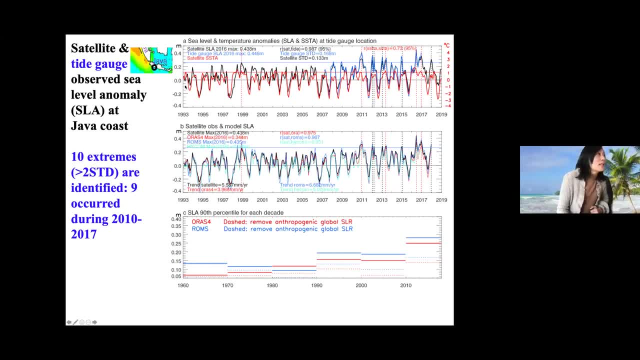 But tide gauge data only have 10 years data, but satellite starting from 1993 here. Okay, So here this blue line. I show the two standard deviation, which is 2.6, it's very, very close to the 90 percentile of this satellite data in the past decade, starting from 2010,. okay. 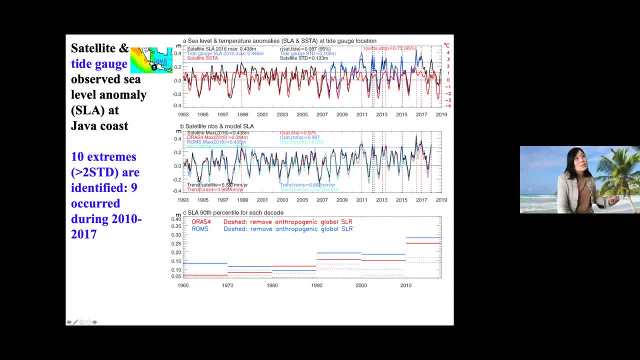 So I'll use this to define this extreme sea level event here. So, based on this criteria, and we identify 10 extreme events as we mark Okay, And this 10 extreme sea level event, 9 occurred in the 8-year period starting from 2010 to 2017, only 1 occurred in 1998.. 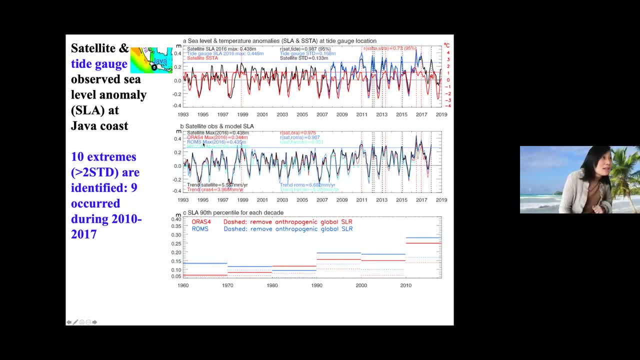 And here this is the second panel I showed- is the satellite repeat, this black line, the satellite data, and here the red line shows again the OIA. as for reanalysis data, which is ocean data, Okay, model assimilated observations, and the blue and the green line shows the purely forward. 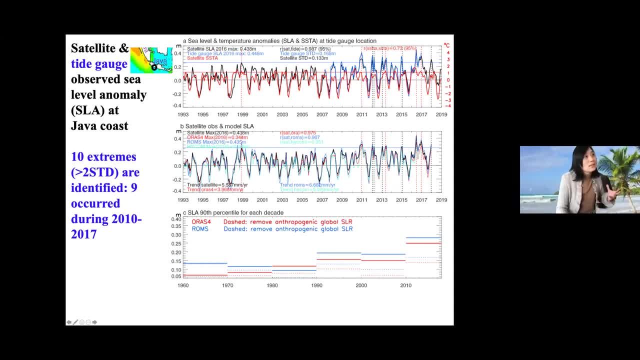 uh two independent ocean general circulation model forced by uh, observed and sort of wind. okay, and all of this agrees so well. why we? i'm showing this because this is a real managed data and the ocean model simulations. we have longer period than this satellite data. okay, so we can put this. 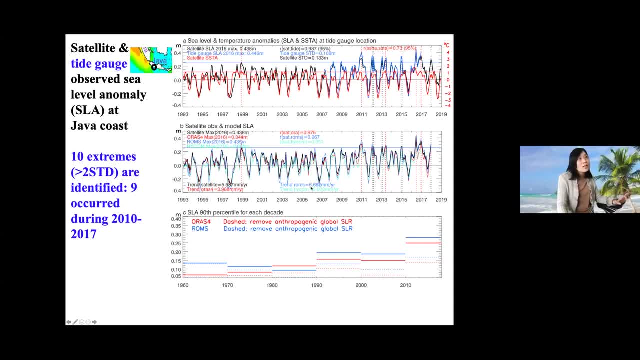 satellite satellite error in a longer term context. okay, all right, this is third panel. i want to. we want to examine what we want to know. okay, how much the anthropogenic warming global- we know that anthropogenic warming causes global mean sea level rise- and how much this. 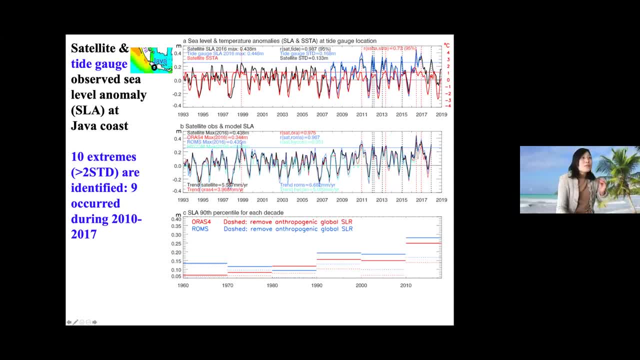 anthropogenic global sea level rise affected this amplitude of the between sea level over the the indonesian area. okay, so to understand that we just what we did is for every single decade, we find the 90th percentile from why? let's look at the red solid line here. that's the 90th percentile. 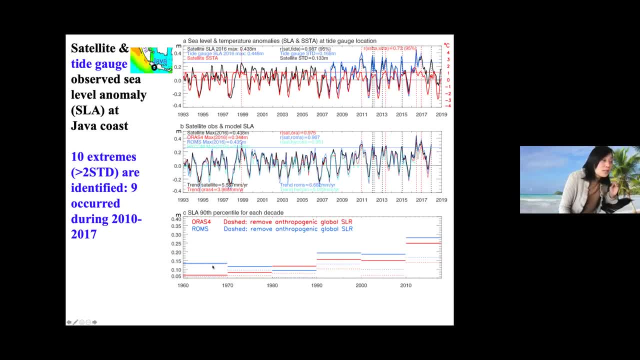 of the amplitude of this extreme of the sea level anomaly. okay, and this is for the 1970s, 1980s, as we can see here. oh, this, or is for sure, persistently increasing the amplitude, but here you do have a down, or a little bit down in the early 2000s, and then you got up, okay, and you have this okay. 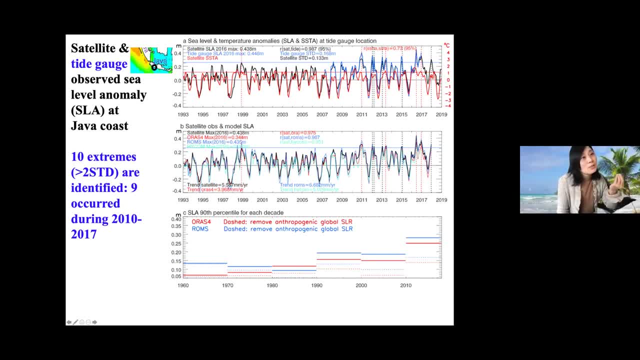 the amplitude, the magnitude of the dream sea level event. yeah, increasing in time in the past several decades. okay, so if i remove, let's remove- the anthropogenic global sea level rise from this data and then do the same 90th percentile, that's the dashed red line. 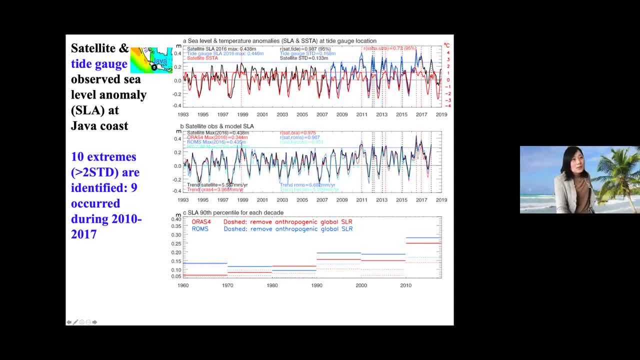 as we see. okay, and that should redline. if you look well, as much dropped by 0.1 meters. what does this mean? global sea level rise does enhance the dream sea level by 0.1 meters. okay, all right, the same thing happened for this. the ocean model. 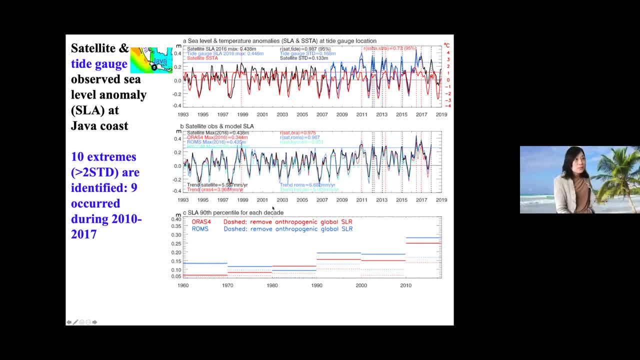 simulation as we can see similar situation, To further show this global sea level rise, on this extreme sea level event. and next I'll show this time series for this whole period of time, but I only show the period of the satellite error to make the figure more clear. 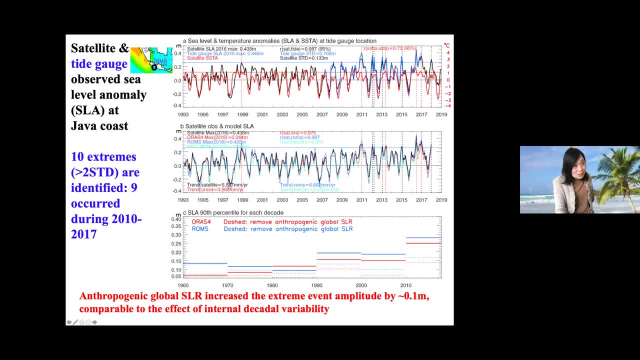 So here we can see this difference between the solid and the red dashed line shows the global sea level rise effect on the extreme sea level magnitude. but this dashed line here, compared with dashed line in 1960s, showed the internal decadal climate variability impact. 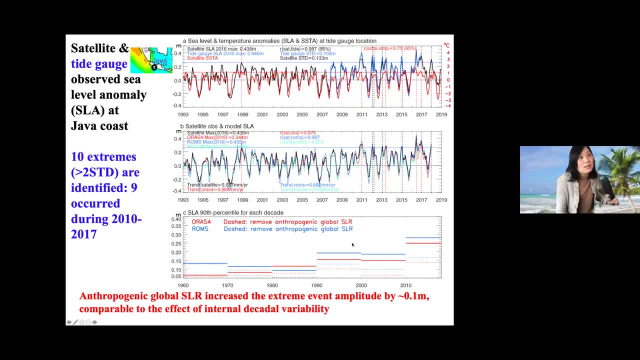 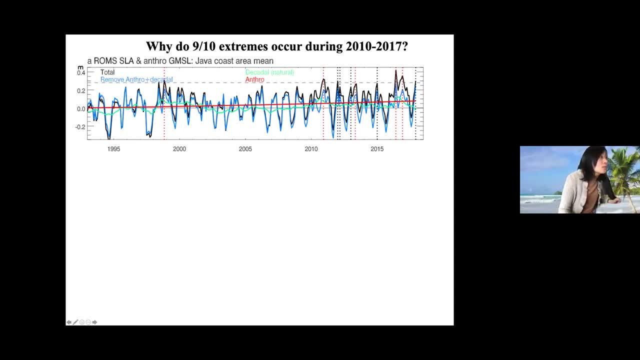 also increased the magnitude of sea level here sea level extreme. So this is a time series. Of course, this is a total from the runs like the ocean general separation model simulation. that's black line, as we showed earlier. agree well with satellite observations, All right, and this red. 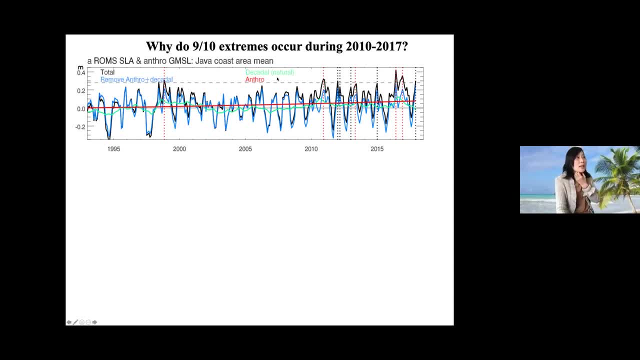 shows this anthropogenic global sea level right. And this blue shows natural we call the internal decadal. climate variability is not forced by greenhouse gases And apparently this blue line is the same as the black, but with these two, with anthropogenic global sea level rise and 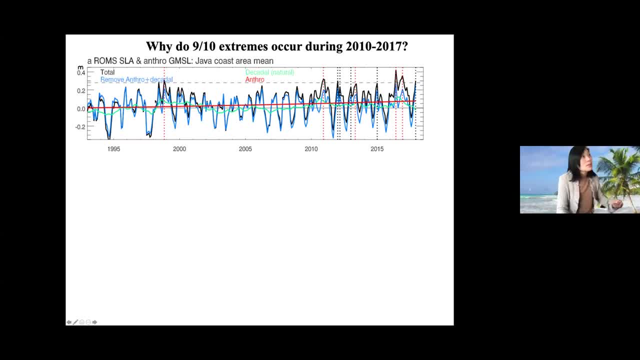 natural decadal variability removed. So if we compare the black and the blue line, we see that, without excluding global sea level rise and decadal variability, this extreme sea level does not have the preference like after this eight year period anymore. as you can see, It does not have. 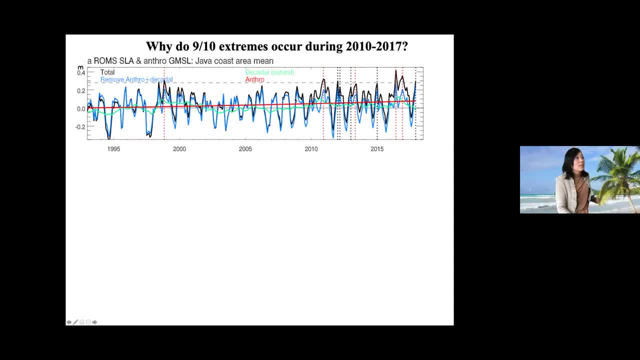 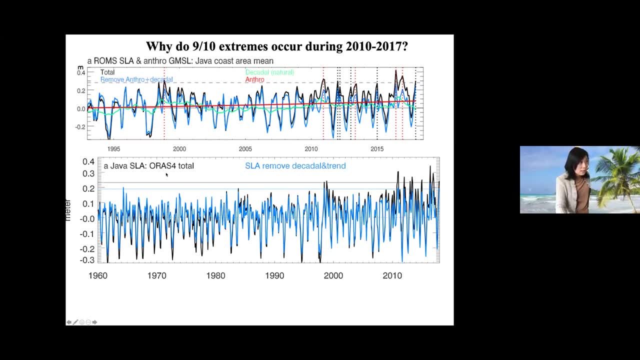 the preference anymore, It's spread everywhere. Okay, this event. Okay, so for a longer period of time. okay, so a lot of Java codes. this is from reanalysis, or I asked for reanalysis data. the same thing. Okay, if we remove the global sea level rise and decadal variability. look at the blue. 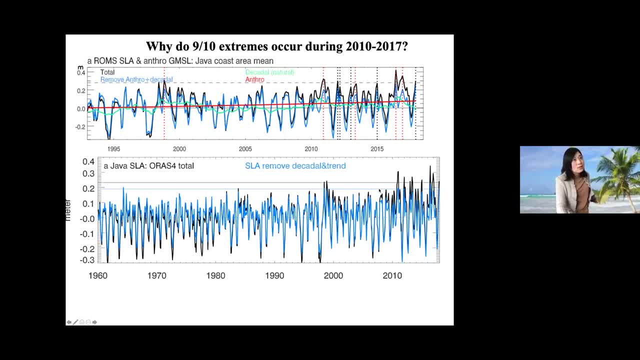 and extreme events. that's not just the concentrated on this eight year period of time, rather is spread out everywhere, Okay, across these several decades. Okay, all right. so this take-home message is that extreme sea level event global, anthropogenic. 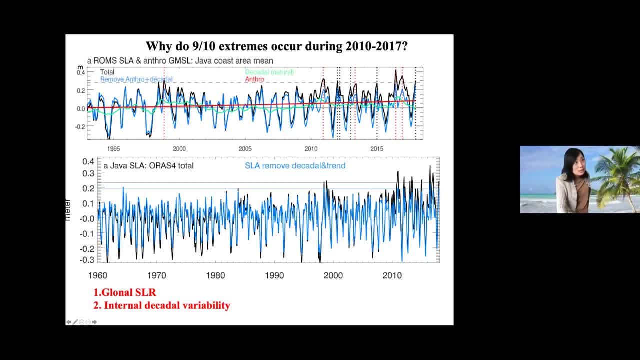 global sea level rise, intensify the sea, extreme sea level magnitude, but the preference of this extreme sea level event that before this eight year period results from two effects: One, global sea level rise intensified right. The other one internal decadal variability. 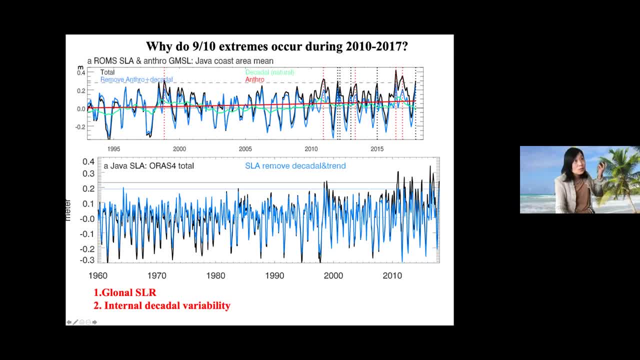 internal decadal climate variability also contribute about 0.1 meter. Okay, so these two together really explain why in the past decade- this in the past decade- basically flooding from 2010 to 2017, that's the most extreme sea level event- occur in this decade- because of these two. 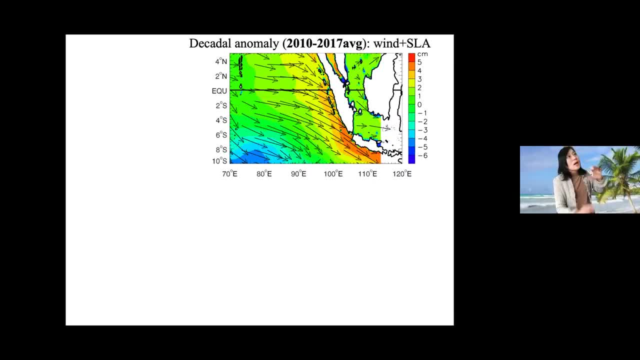 factors. Okay, and so how? the decadal variability intensified in that decade intensified sea level along the Indonesian coast in that during that decade. So here I show the sea level anomaly, which is color, and the wind anomaly, averaged during that decade. Let me hide that floating bar. 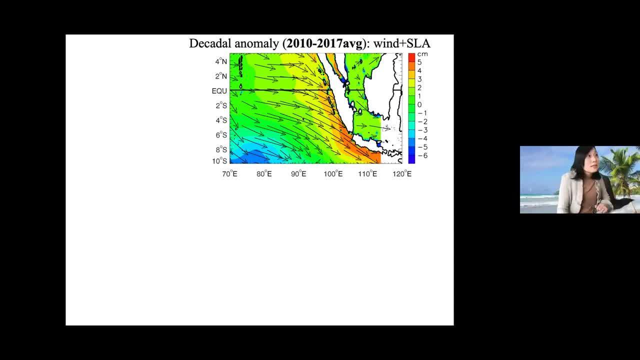 Okay, all right. so here and we see, we explained earlier, this westerly wind really piled up water to the eastern boundary and when they impinge onto this Sumatra coast and the signal can also propagate forward. Meanwhile, look at this- a longshore wind, This longshore wind, if we should call. 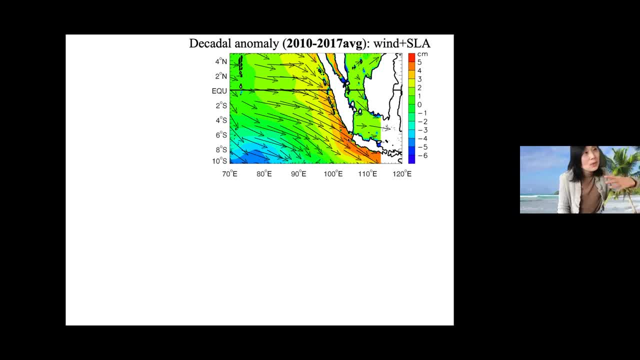 and causes the ocean surface water to 90 degrees to flow: 90 degrees to the left. Okay, so that converts to the coast. Okay, so you convert or push all the warm water to the coastal area and increase the sea level. Okay, so this is both the local longshore wind and the equatorial wind contribute. 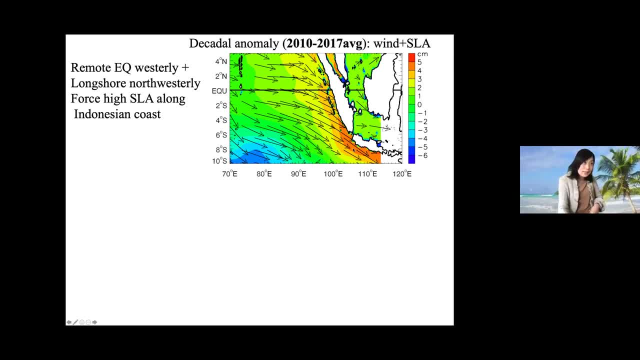 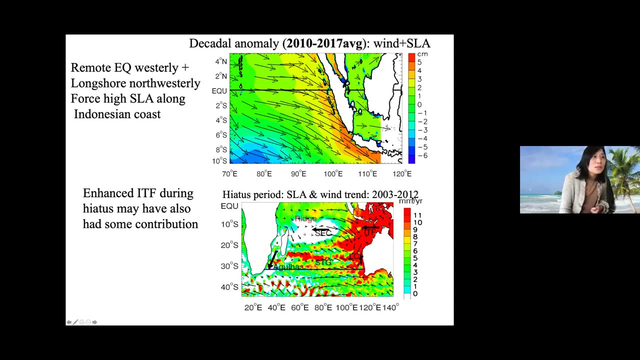 to this increased sea level during that decade, which boosts up the frequency of the extreme sea level event, together with global sea level rise. Okay, and here we focus on the Indian Ocean and, as we know, from 2003 to 2012,, that's, we have intensive 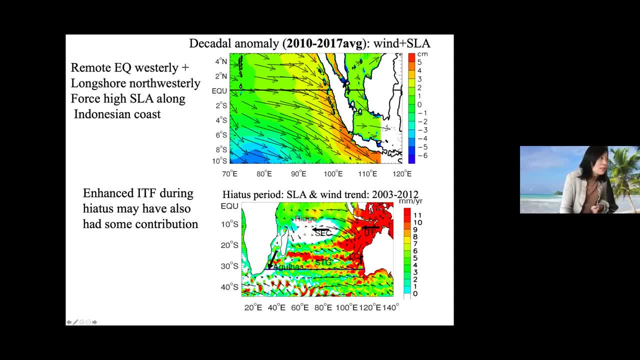 climate change in the Indian Ocean. So we call this global surface warming hiatus period. We'll discuss next. So this may also contribute a little bit and bring the sea level a little bit higher from 2003 to 2012,, although this only cover a little edge of this period. 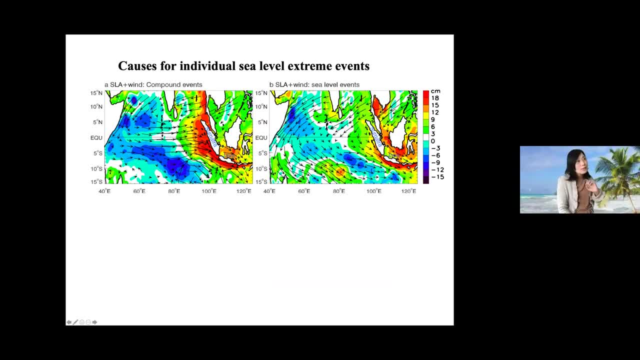 All right for individual sea level extreme events. I do not want to discuss too much, but this one I show the surface wind pattern associated with individual- Okay, extreme sea level event. this one also co-occur with marine headwaves. This one only extreme sea level, as we can see. 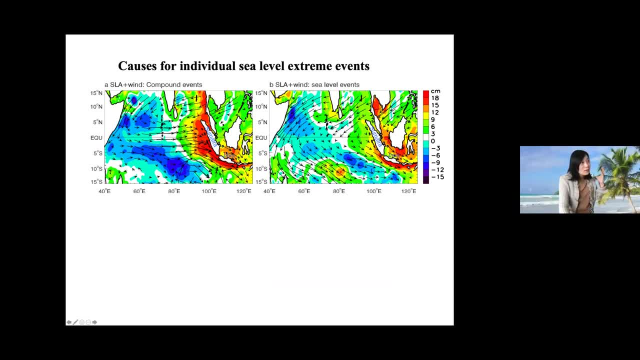 strong equatorial wind and the longshore wind at a kick cost for this extreme sea level event at inter-annual time scale. Okay, and this one only. local wind play more important role. But for here I do not discuss the details, but here we have a manuscript, If anyone. 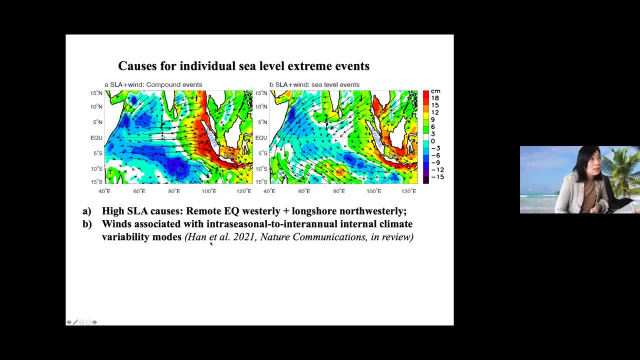 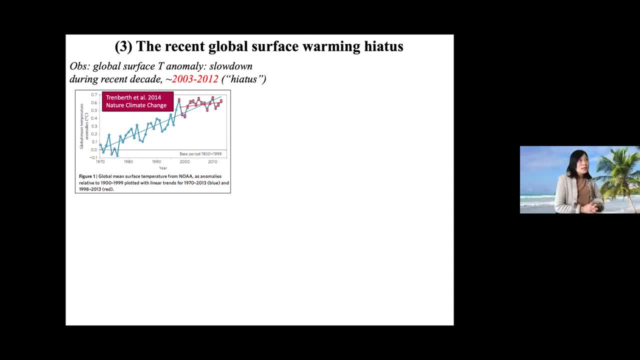 want to discuss further. you can always reach me after the talk. Okay, so we just mentioned that there is a global surface warming hiatus period. okay, from 2003 to 2012.. What is this hiatus period? So we showed in this first slide, as we introduced because of greenhouse gas increased. 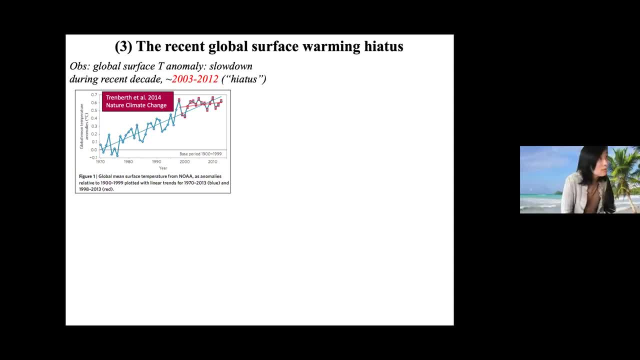 greenhouse gas concentration in the Earth's atmosphere trapped heat, Okay, so it increased the sea surface temperature and warmed the ocean. So this is the time series of global surface temperature, including surface air temperature and sea surface temperature, Okay, starting from 1970s. 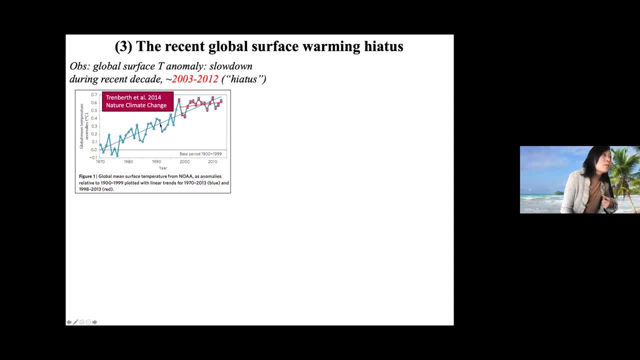 as we see going up up. okay, warming as we see this Earth's surface warming, but if we look at this decade, it's from 2003 to 2012,. almost flat, Okay. so here and this surface, the global surface. 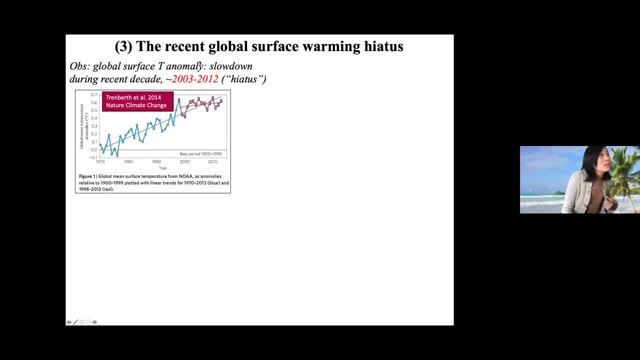 did not show the warming. It seems like stopped. That's why it's called hiatus. Okay, it's hiatus, flat getting flat. here We didn't increase. But if we look at global mean sea level, continuous increase and accelerated increase sea level, Okay here. So, as we know, this is only surface temperature action. 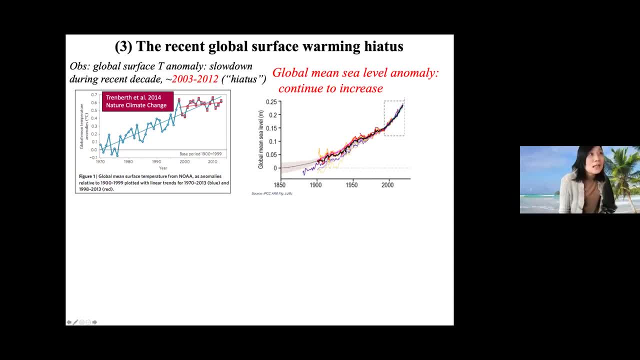 Okay, but sea level, what does the sea level represent? The vertically integrated feature of the whole water column column of the ocean, All right. so if we have the warm water convert in the water column, we increase sea level Only. sea surface temperature increase may not cause a. 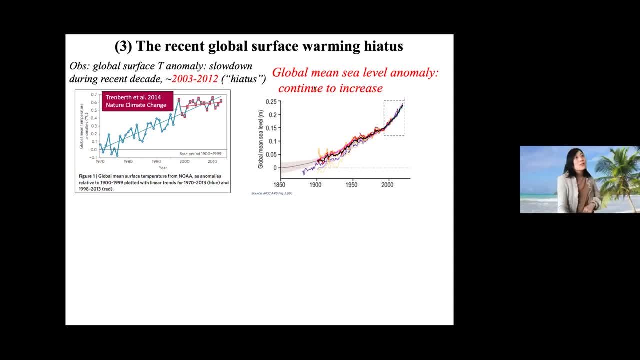 sea level increase May or may not. Okay so, because this one represents whole water column and this one only represents surface. and then we know, during the same period of time, greenhouse gas is still trapped, continues to trap heat in the Earth's climate system. Okay so, we still have excess heat in the 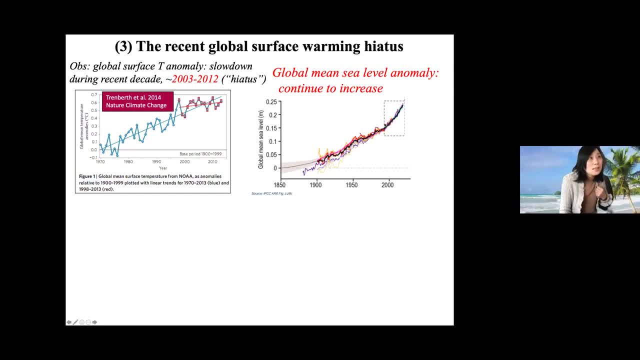 climate system and surface not warming, but the sea level keeps increasing and the sea level represents the whole water column. What does this mean? This means that excess heat increased is stored in the subsurface ocean. Okay, so increased subsurface ocean uptake is the major sink. 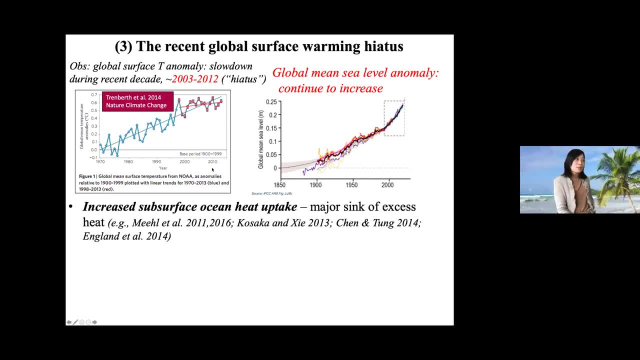 And so now look again here. So this is a good point outlined here. So instead of a stay, you can concentrate most of the heat went and continue- sufficient heat to escape. Also, more and more subsurface ocean has increased and the surface temperature. 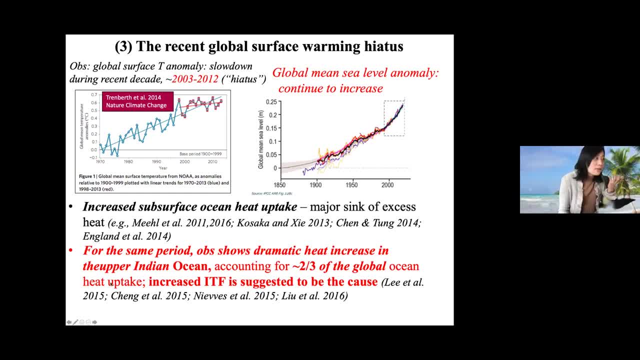 is also increasing. So, through the discussing process, only springs are entering this part of the ocean. However, be aware that this will not cause any wonderful advising. That means doing something Haeitg instead of making undergoing operations, So we'll talk more about this. 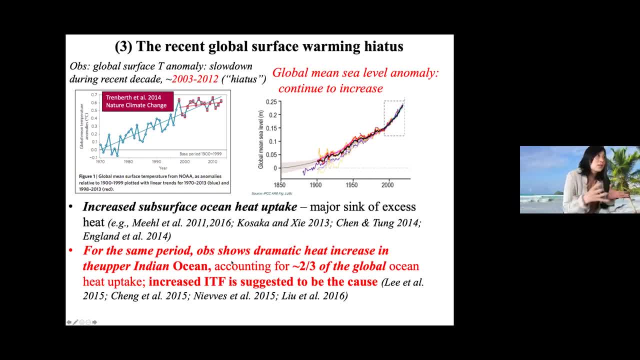 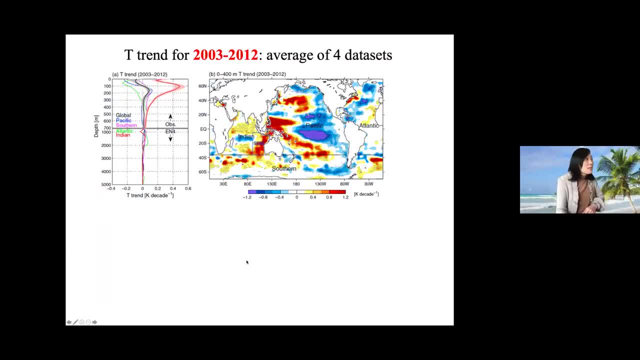 briefly, ocean circulation from the pacific to the indian ocean through this indonesian through flow. we call itf right, so here, and to further demonstrate that, so here, as you see all those lines and that's the average temperature at the surface and at different levels, and and to the five southern 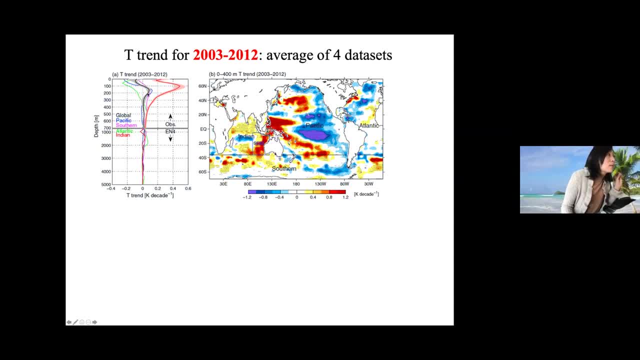 meters. okay, global average is the black line. global average as surface, as you can see, is negative cooling if you average surface temperature, uh over the globe. but the global average, the temperature in the summer surface from 100 meters to 400 meters is warming, further demonstrated that the heat is stored in the surface of the ocean. but if you look at atlantic, 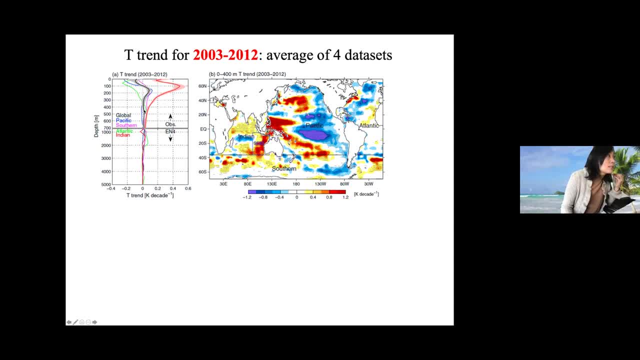 to tell the temperature here, and by relative temperature you can answer that okay. and then this: let's say: temperature is digital here. so, um, the temperature at supert Melt, which is green, okay, it's cold after ocean, okay, in deeper part a little bit warm here, but a southern 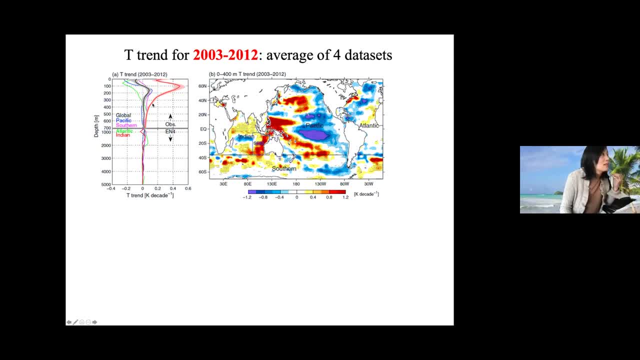 ocean called the surface and here super surface ocean also showed okay, increase the heat storage. but the maximum pacific shows a little bit as well. the maximum dramatically increase of heat is over the indian ocean. okay, just like the previous study show here. okay, in the upper 700 meters, especially in the upper 400 meters, as we can see right. so the right panel shows the. 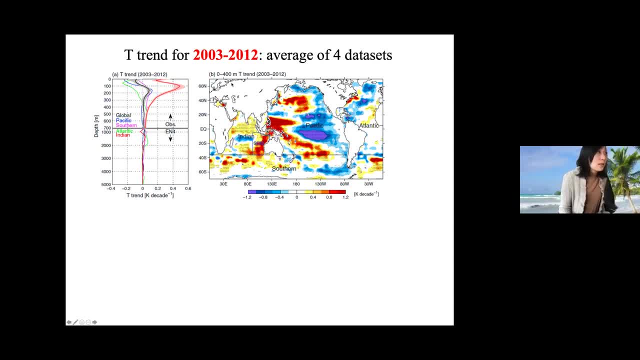 visual the pattern of the trend for this hiatus period in the upper 400 meters. okay, uh, temperature trend in the upper 400 meters represent ocean heat content in the upper 400 meter and apparently the heat is stored over the indian ocean, which account two-thirds of the global heat storage. 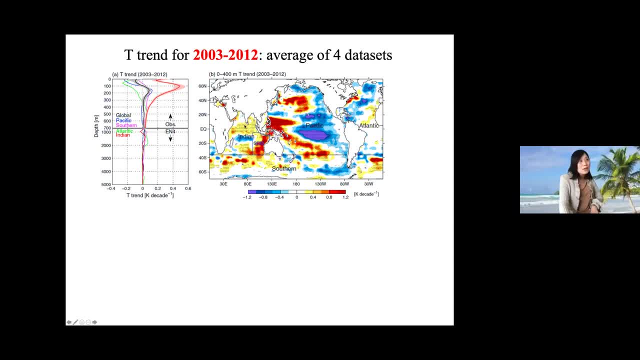 primarily stored in the southeast, in the ocean, although in the equator, and here also have sun, and this southeast indian ocean, here is strong, most of heat, there's a heat concentration in this area. okay, because of this, and the temperature, uh increase here. that zero point, zero point. eight to one. 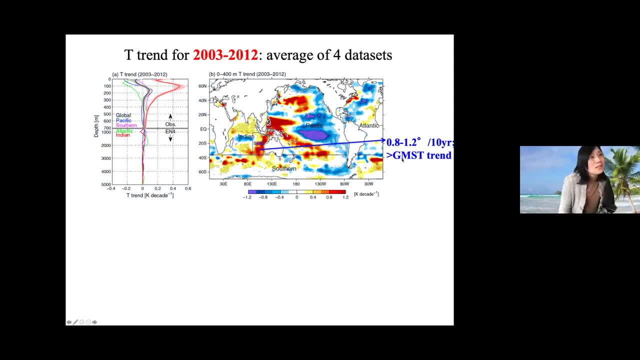 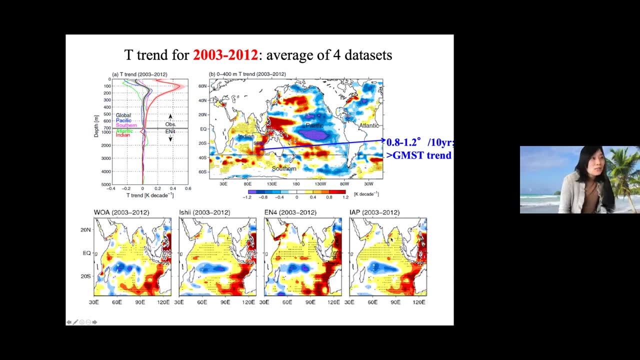 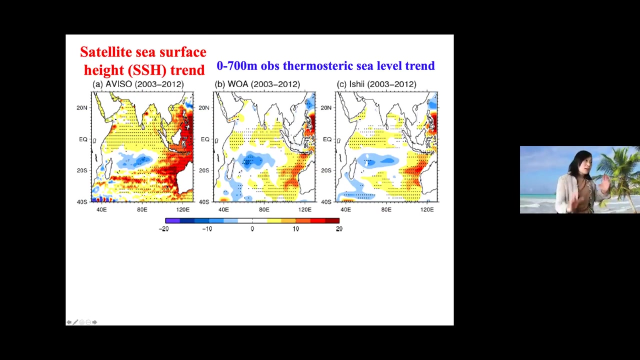 point: two degree percent uh per decade, which much higher than the global uh warming trend. okay, and this pattern occurs in all the different ocean in situ observational based ocean uh temperature data set. okay, and suggesting the robustness of this uh pattern. as we mentioned before this, if you have a upper ocean heat increase in a specific area, it must be reflected. 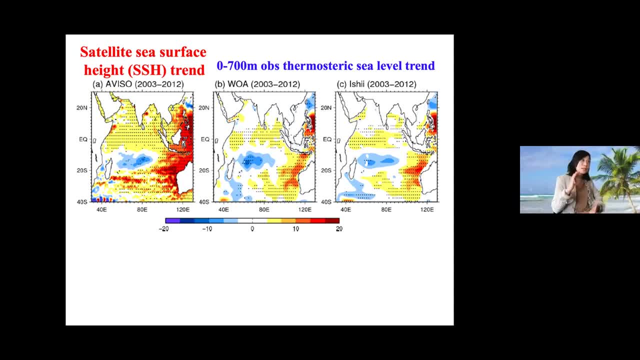 by the sea level, because sea level represents a vertically integrated uh feature for heat, fresh water and mass. okay. so apparently that's the uh. we have the high sea level here. okay, strongest sea level rising trend in the southeast indian ocean at 16 centimeters per decade. decade 16. 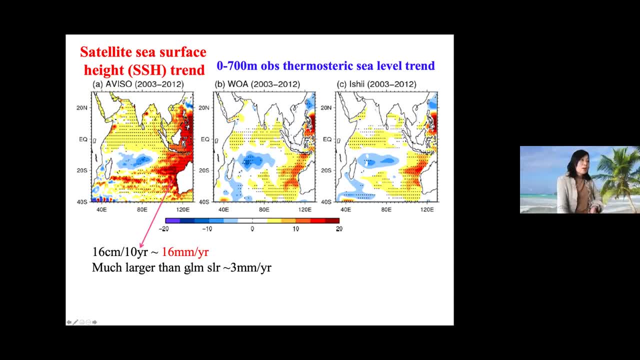 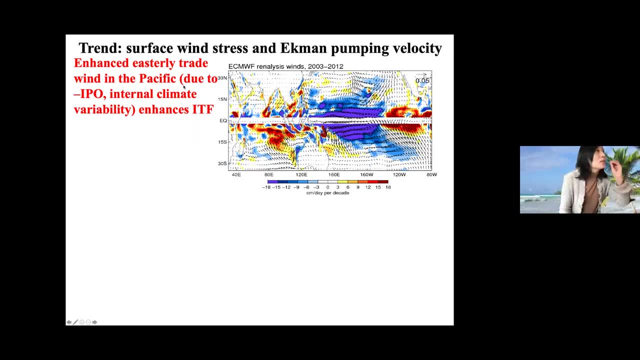 millimeters per year, which is much higher than the global average sea level right rate. all right, here i we won't go to the further detail. this is a surface wind trend. we try to understand why there is increased through flow, increased heat and the threat heat and the warm water transport. 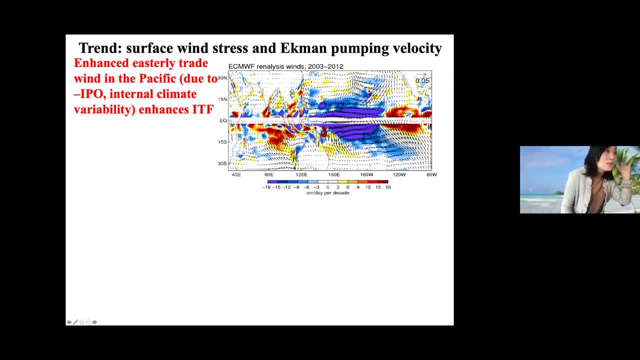 from pacific to the indian ocean and why it's confined to the southeast in the ocean. this is the sea, uh sea, surface wind. as we can see, the trend shows strong easterly trade when the intensified is retreated i mentioned earlier, and this intensified is retreated when 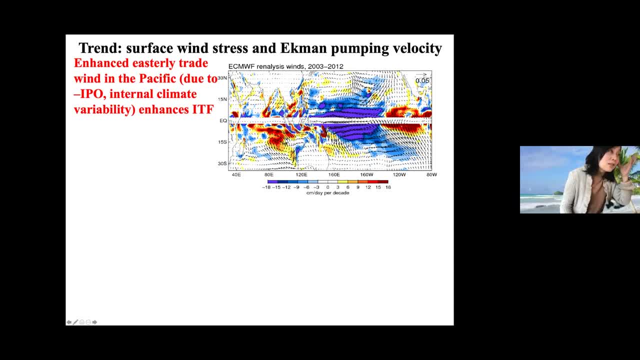 the power of water in the western pacific enhanced, you know, eastern through flow, and it's transported into the indian ocean, okay, and after interacting in the ocean. this is clockwise, when the pattern, as we see, confined this water to the southeast in the ocean, if we still recall, if the wind blew from. 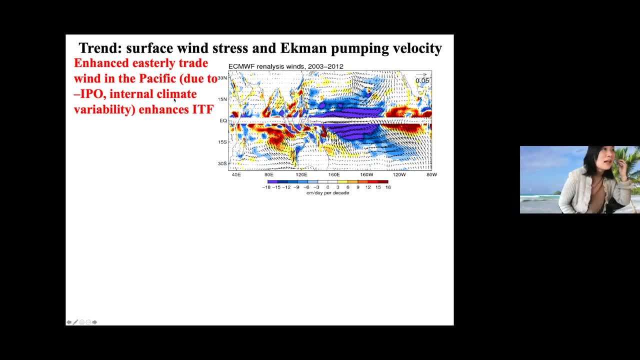 the north to south in southern hemisphere and the surface- uh water we call the surface element transport is 90 degrees to the left. so it should be 90 degrees to the left when it should be onshore. so you accumulate the warm water onshore, you increase the sea level, increase the heat content in this area. okay, so where is this? 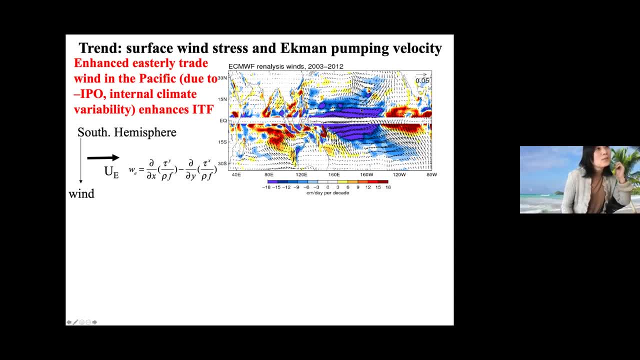 intensified uh, uh is retrieving from, they said, this part of this uh, internal current variability, the negative phase of inter-decadal pacific oscillation. So here you do not need to know, you just need to know. during this decade you have intensified this event due to the internal 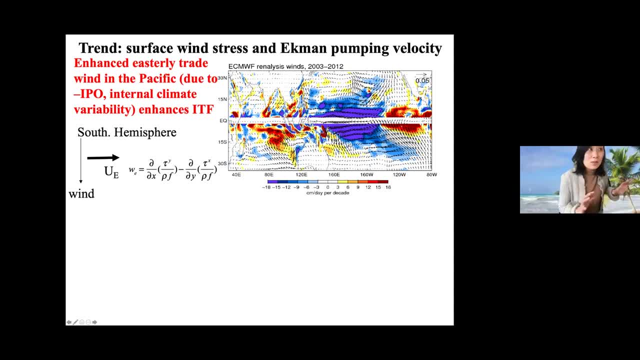 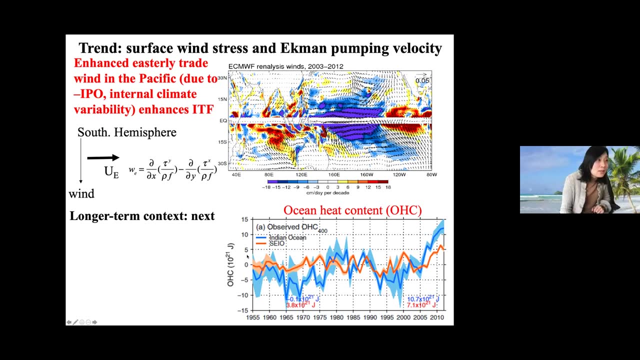 climate variability, And this internal climate variability redistributes the heat associated with greenhouse gas warming in the climate system. All right, to put this hiatus decade into a longer-term context, we show the upper 400-meter ocean heat content over the Indian Ocean blue and in the southeast Indian Ocean. 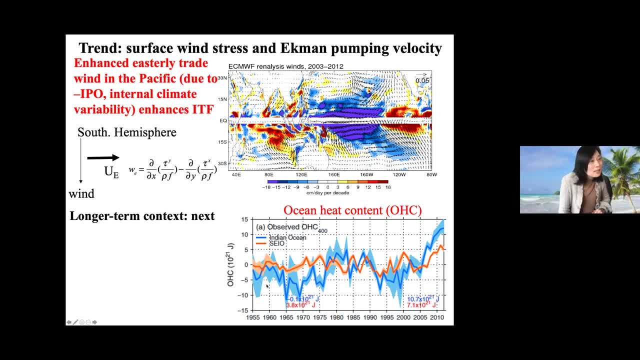 area. okay, as here. apparently, we see an upward trend Overlying the upward trend. we have decadal or inter-decadal variability and there is intensified decadal variability in this hiatus period over both the whole Indian Ocean and the southeast. 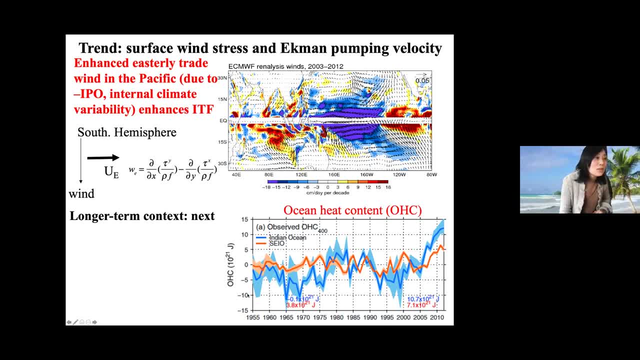 Indian Ocean. okay, So, even though part of this upward trend might be due to insoluble genic warming and part due to internal variability, but this can be intensified by internal variability. Okay, so the ocean heat content during this hiatus period in the southeast Indian Ocean account for about 66 percent. 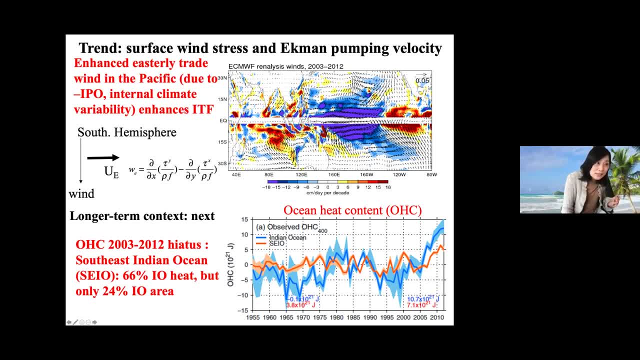 of the entire Indian Ocean heat content increase and its area is only 24 percent of the Indian Ocean, suggesting that the southeast Indian Ocean of the west Australian coast has a strong heat increase. rapid heat increase in this area. okay, So the rapid heat increase. 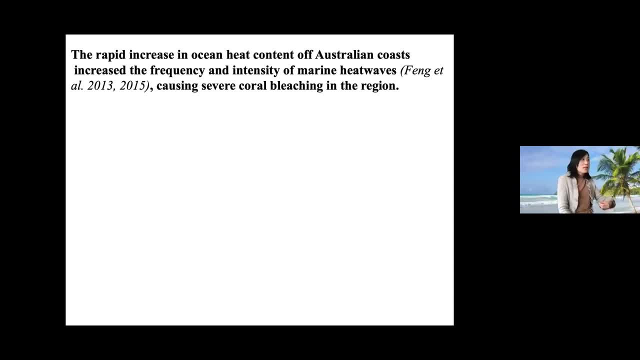 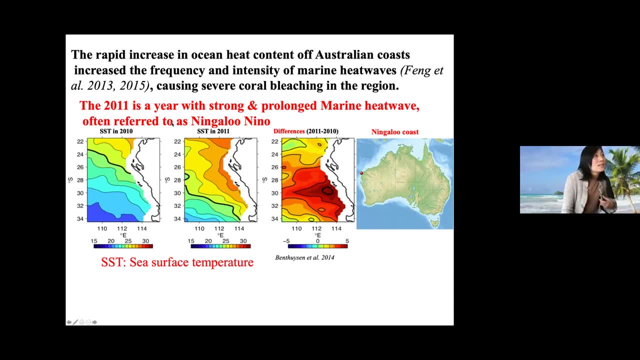 in the ocean heat content of the Australian coast increased the frequency and the intensity of the marine heat waves. okay, as suggested by existing studies, that causes severe coral bleaching in the area. So this is a sea surface temperature plot as we see in 2010,. 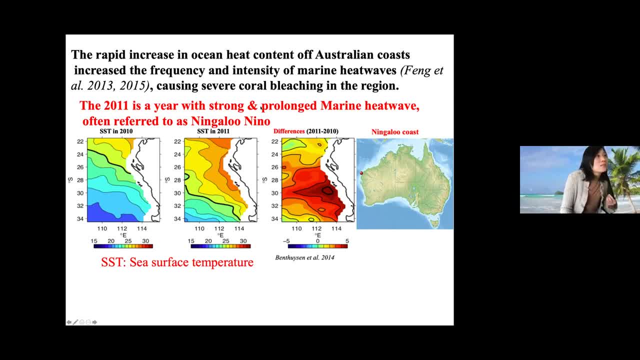 and this is in 2011,, which is a year of strong, prolonged marine heat wave. okay, Some research articles show called this Ningaloo, you know, because Ningaloo that's the area, that's the location here, right off the western Australian coast here. okay, So that this is the difference. 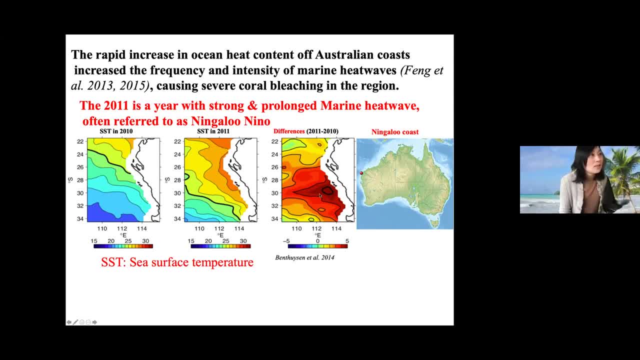 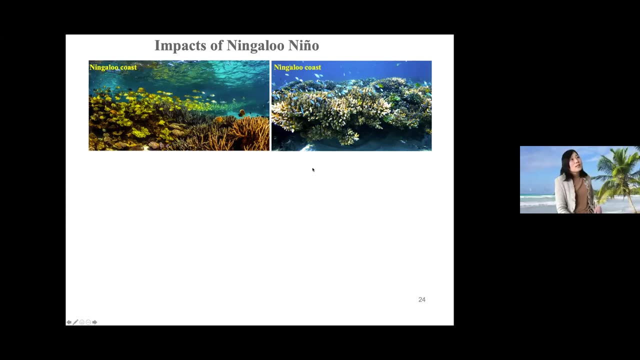 between 2011 to 2010, sea surface temperature. as we can see, in some areas sea surface temperature increased by almost four, three to five degrees. look at here: okay, So this is a strong temperature increase and the marine heat waves and intensified by the increased. 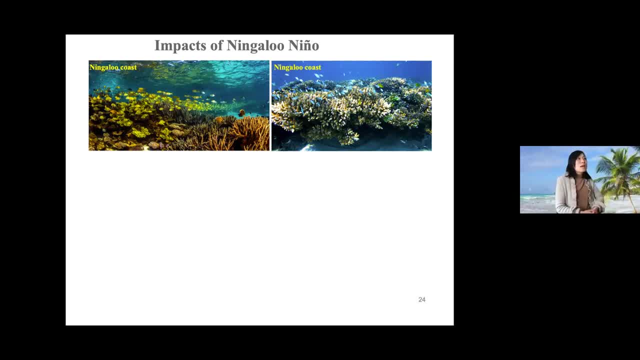 becadal-scale ocean heat content have a large impact on the marine ecosystems. So this is the Ningaloo-Ningaloo coast, which is very nice and has diversified of the marine species and also its habitat, its habitat to many, many marine species here. But during this 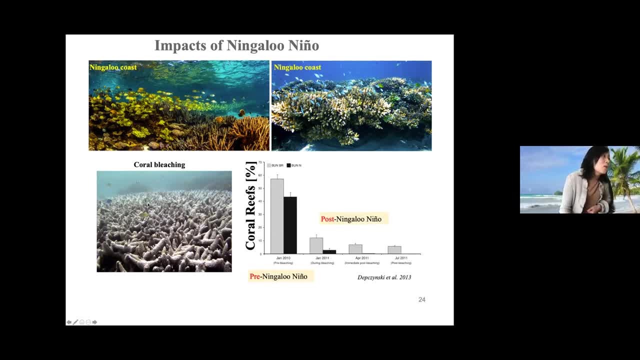 heat waves, like we discussed 2011,. the corals have bleached okay, So here they study, the two areas near the Ningaloo-Ningaloo area they call Marine Park. and two areas, okay, This one gray. 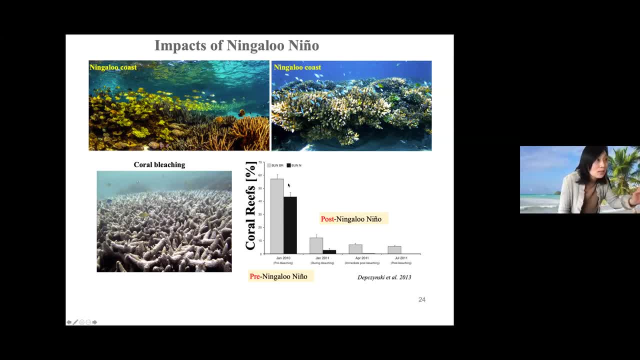 represents one region, the other, like black, represents another region, and just two study sites, okay, only two kilometers apart, and they both at two to five-meter depths. they measure this area okay, The cover area of coral, live coral, okay, And so what we see the pre. this is the pre-2010,. 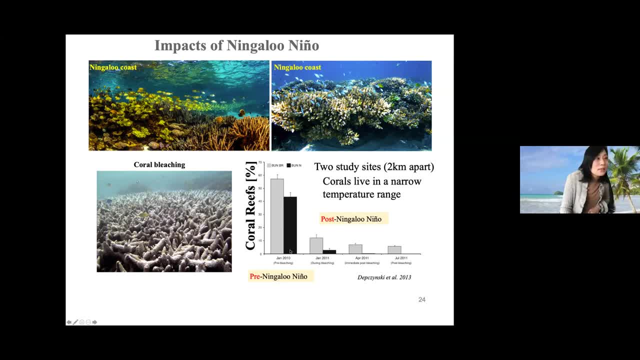 that's pre-bleaching the pre-marine heat wave event. look at this: the cover almost it is 57 or 58 percent area and here cover 45 percent. But during this January 2011 marine heat waves. 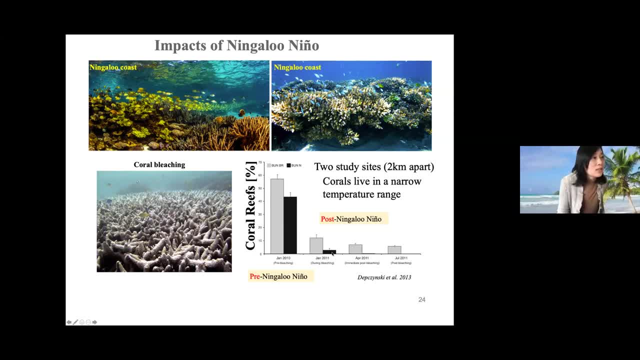 look at this: the live corals dramatically reduced. and here, dramatically reduced. But a few months later, after the post, immediately after these heat waves, look at this black. the second area: it's about zero, almost gone, all gone, okay, Eight months after this heat wave event, 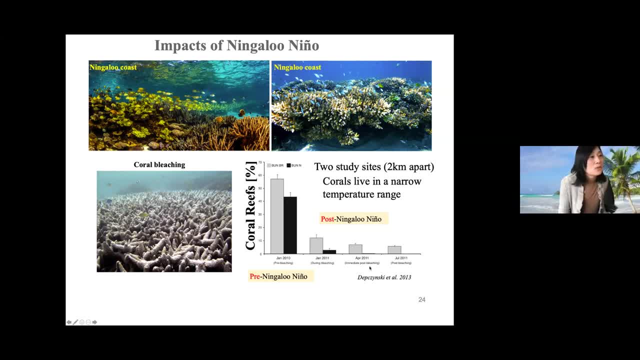 this black second area completely gone, like all the corals died right And here, only one to 60 percent the first area, only one to 60 percent corals alive. okay, All right. so in summary, and the first part: 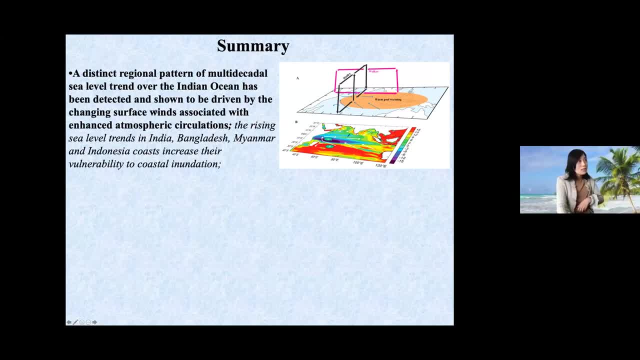 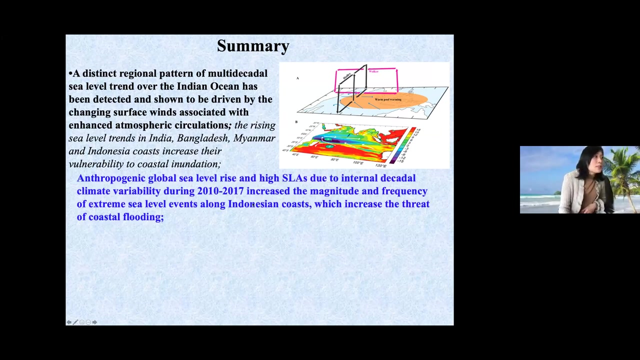 we show a distinct regional pattern of multi-degenerate sea level trend over the Indian Ocean and this is due to the intensified atmospheric circulation. So the rising sea level trend in India and Bangladesh, Myanmar and the Indonesia coast really increased their vulnerability to coastal inundation, Encyclopedic global sea level rise and high sea level anomalies. 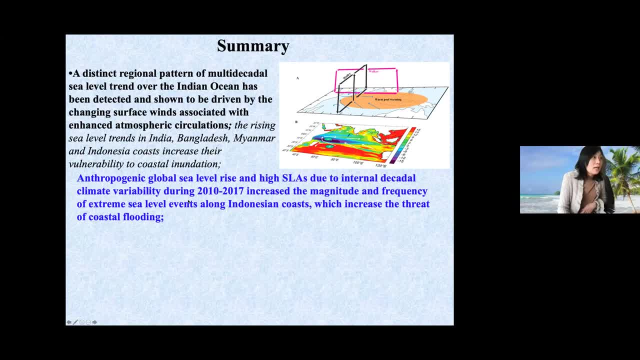 due to internal climate variability And, for the eight-year period, increased magnitude and the frequency of dream sea level event along this Indonesian coast, which increases threat of the coastal flooding in this area, plus their sinking, fossil sinking- of their land. Lastly, the rapid 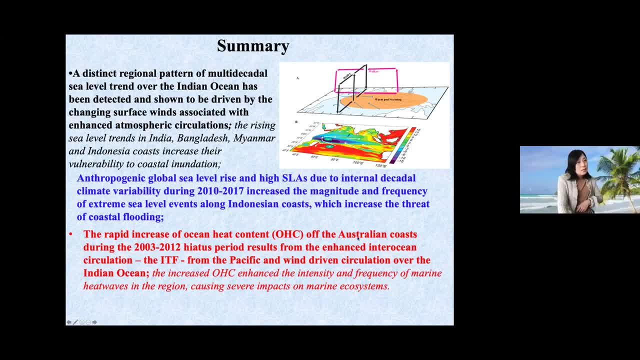 increase of ocean heat content of the West Australian coast during this recent hiatus period and results from the enhanced intra-ocean circulation that's intensified the Indonesian flow from the Pacific and the wind-driven ocean circulation that can find to the Southeast Indian Ocean And the increased ocean heat content enhanced the intensity and the frequency. 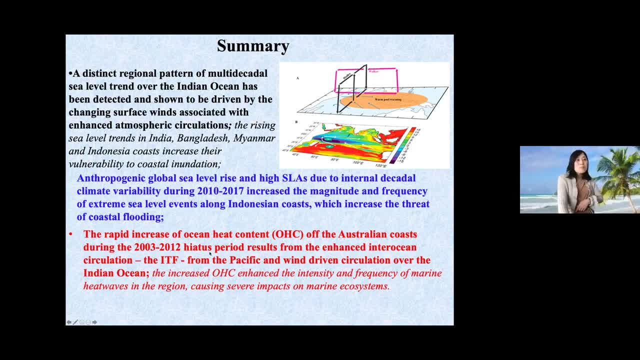 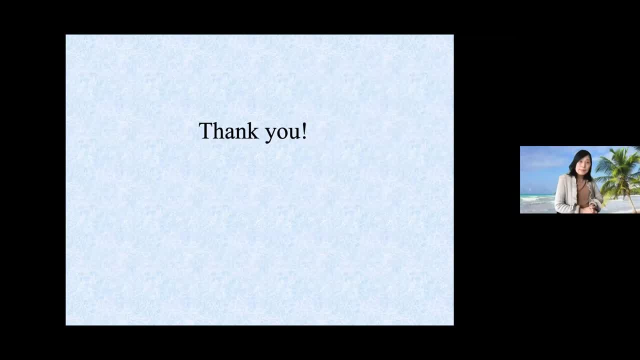 of marine heat waves in the region, causing severe impact on marine ecosystems. Thank you, What's wrong? Thank you very much. Thank you, I hope you could hear the clapping here in the room. Maybe you could not hear it, but there was a lot of clapping. Thank you very, very much. 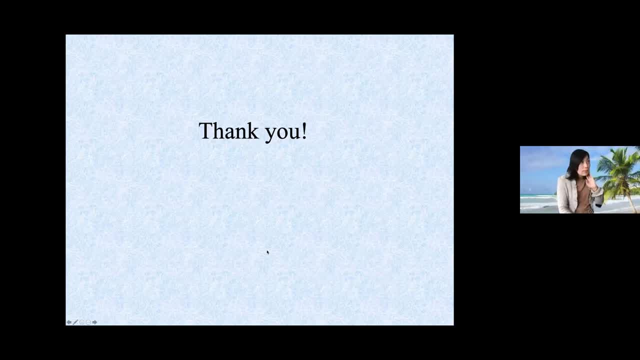 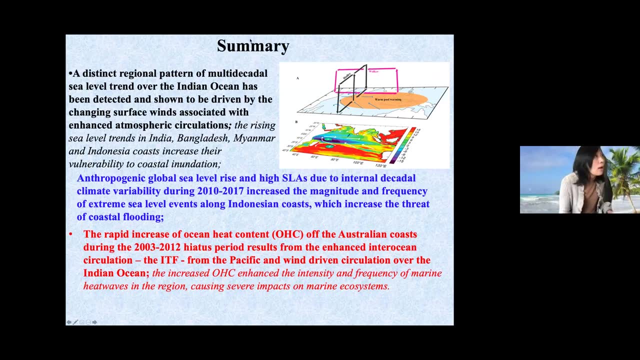 So we have a lot of questions already I see in the chat. So I don't know if you can see the chat also yourself, but I will. in any case I will read the question so that everybody also can hear it. So we have a question from James. 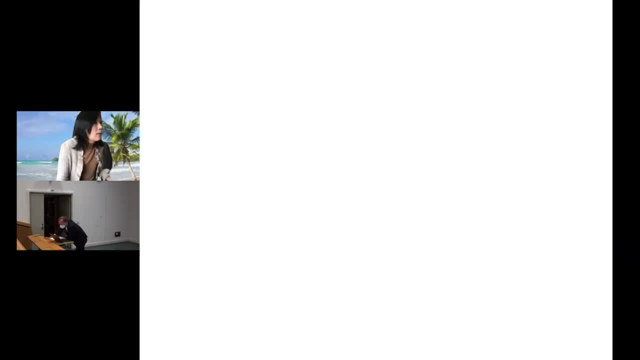 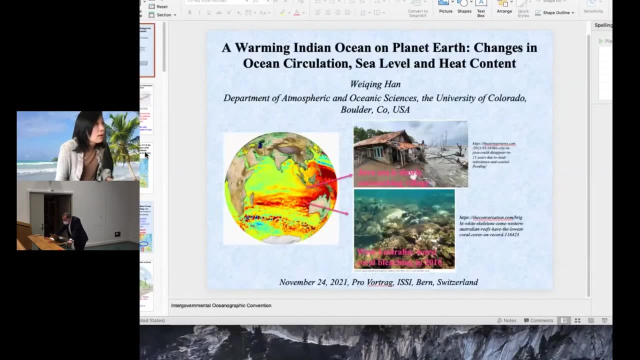 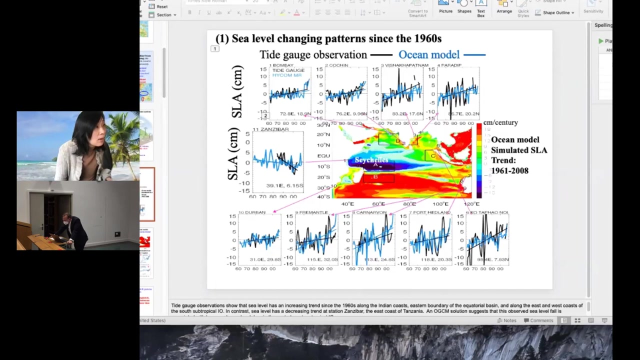 Lord and he writes hi there. I'm not sure if you're taking questions via the chat. If they are, I would like to ask this one: Do these patterns in sea surface right anomalies persist throughout the year, or are they times of the year when the anomalies become more or less pronounced? 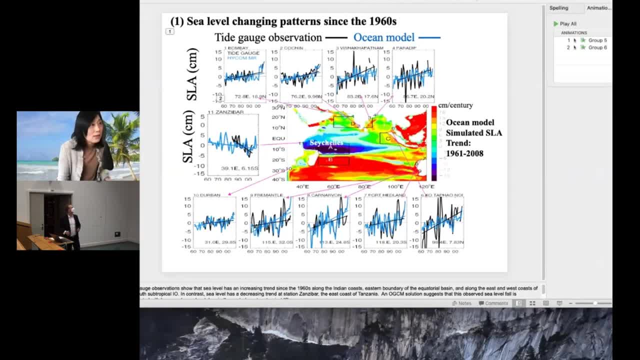 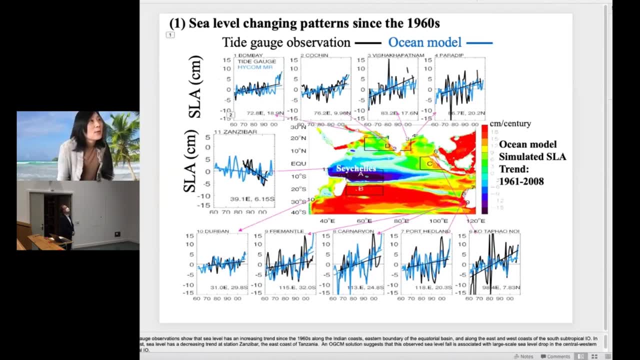 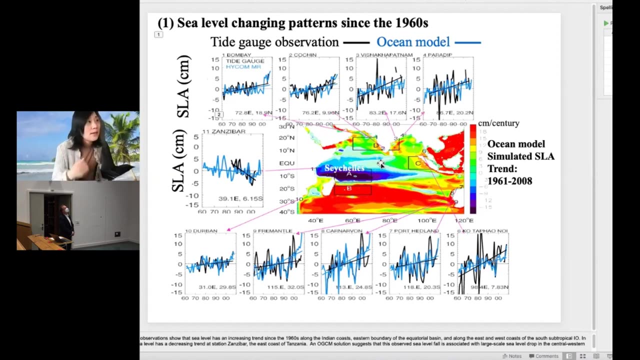 Oh, that's an excellent question. Okay, very, very good question. We did do this. I showed here it's the annual mean And we did explore the south-east. We did explore because the Indian Ocean is subject to monsoon, seasonal, very seasonal, okay, So summertime and the wintertime. 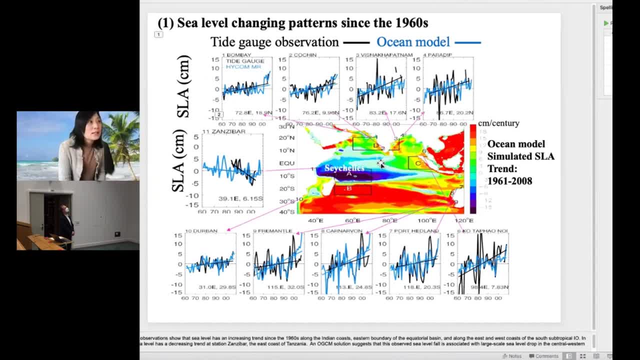 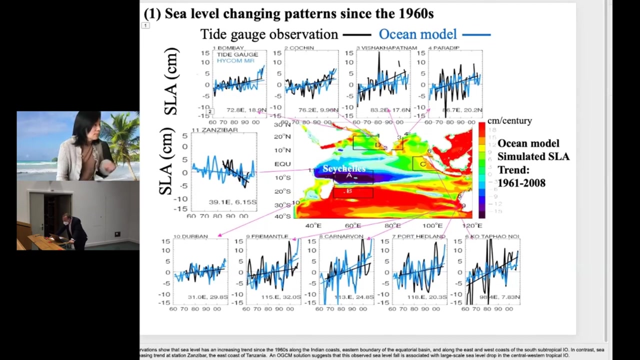 And I think the, if I recall correctly, the wintertime has a stronger inundation than the summertime. That's the monsoon season. okay, That's an excellent question. That was a second question. Do we see similar patterns in the Atlantic and the Pacific as in the Indian Ocean? 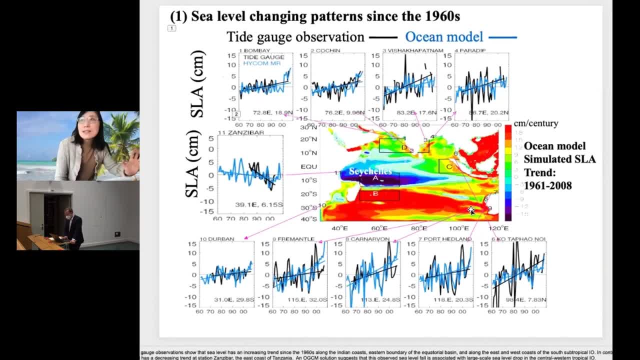 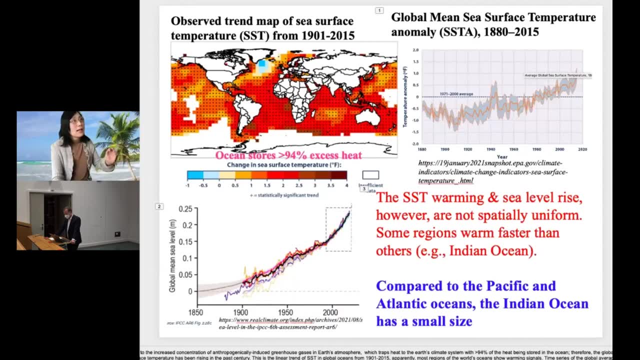 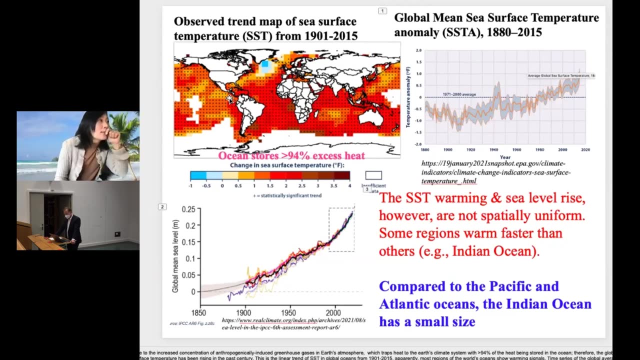 Oh, another, that's another excellent question. I recently, oh, I didn't understand, those didn't bring that. but let's see, let's see this one. Okay, the first one. you look at that and this is one thing. that sea level pattern, I didn't. I only look at this. we are working on some. 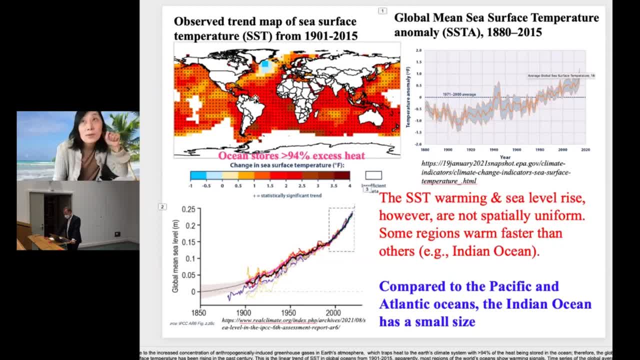 US East Coast sea level. Okay, so in the past few decades we there are extensive- I can't say extensive, but quite a many research discussing the rapid sea level rise along the US East Coast and there are a lot of speculations. Climate model simulation show that. 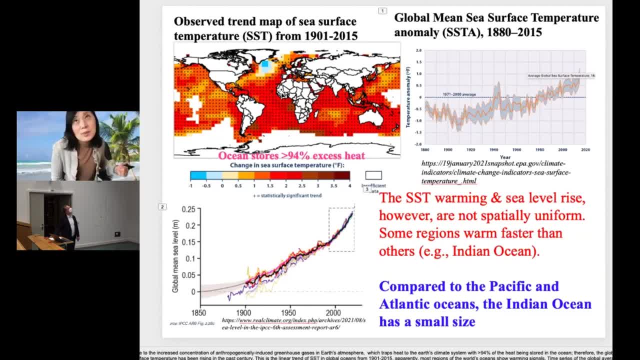 if you have. we know Greenland ice sheet has been melting faster since the 1990s. right, and some people say, oh, because the Greenland ice sheet melting, you dump fresh water, reduce the Atlantic meridian or three and a. 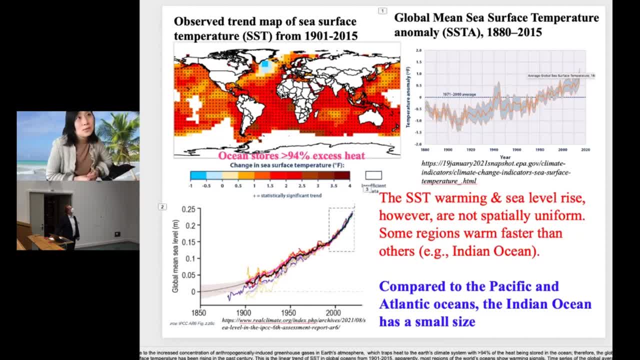 third of the ocean population. you have a dramatic increase of US East Coast sea level and some idealized model experiment using climate model did show that. but there is recent, I think, 2016,. there's a high resolution model simulation work by Klaus Brumming and he showed that the melting Greenland ice 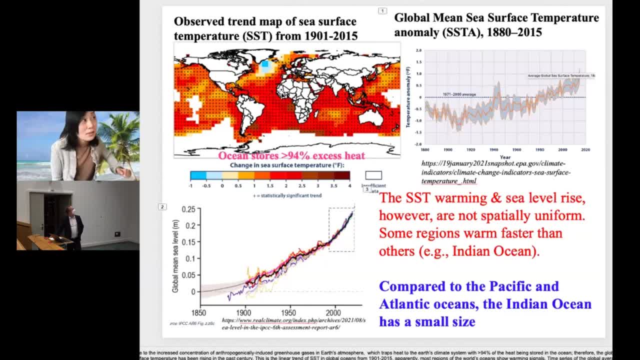 sheet water has not yet reached this US East Coast. This is still active area research. By the way, if you look at this sea surface temperature, it is active at the active area of Greenland ice sheet. This is an actual survey of data from the Greenland ice sheet at least two years ago and this, this is a. this is an accurate 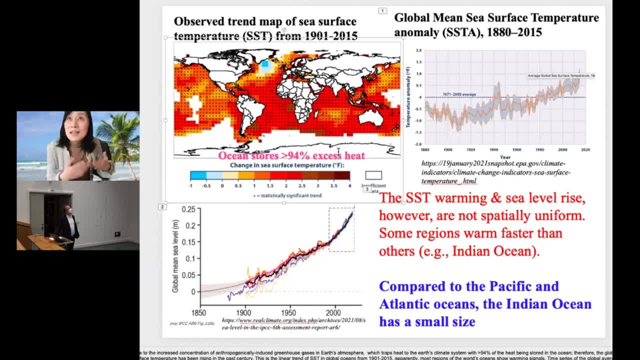 analysis and also the kind of social function at Greenland ice sheet is the same. So in the PNAP here you can see, in the PNAP you can see the rise of the PNAP or the rise of the PNAP. 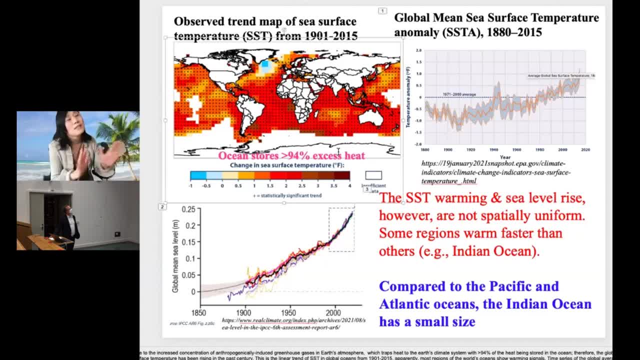 and the rise of our PNAP, and it's not, and this is the same. so that's on the side. so you can see the rise of greenland ice sheet here. Now, if you are, if you have any questions about climate and the climate relating to ice sheet, I think you get the 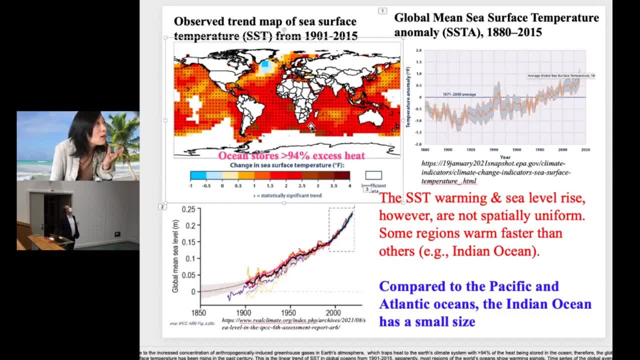 The Indian Ocean. if you see, you can see overall warming faster than the central and eastern tropical equatorial Pacific Because the warm Indian Ocean and cause atmosphere response and you cause easily treatment in the Pacific Ocean. This easily treatment intensifies the cold water up well to the surface, which they call thermostat mechanism. like counteract the surface warming a little bit. 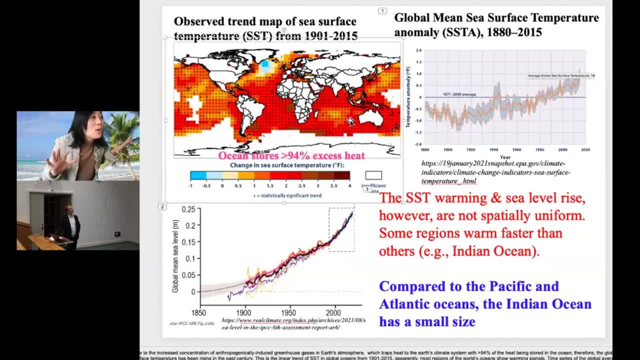 So maybe the Pacific in the global warming sense- and warming is not uniform everywhere as well- maybe the warming Indian Ocean slow down the tropical equatorial Pacific cold-town warming, But still there might be some people disagree, but still active area of research. 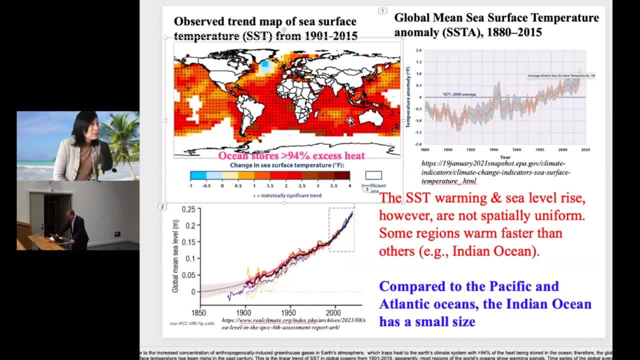 Excellent questions, Thank you. There is a further question from Paul Temme, And he writes: thank you very much, King Han. My question is: does the ENSO circulation have an influence on the Indian flow-through? Oh good, Yes. 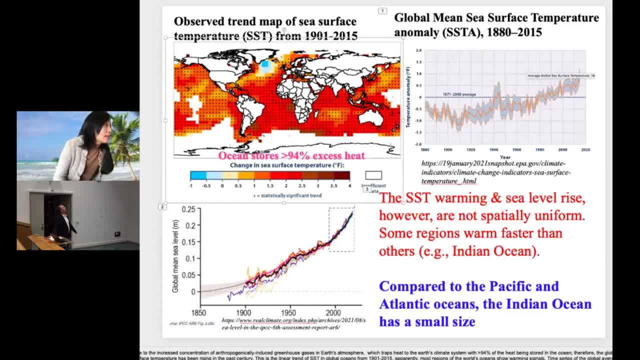 ENSO does. Let's see. Let's discuss this hiatus theory. Let's look at it. Yes, ENSO- tropical Pacific Ocean circulation. the most dominant mode we all know is ENSO. Yes, ENSO- tropical Pacific Ocean circulation. the most dominant mode we all know is ENSO- Yes. 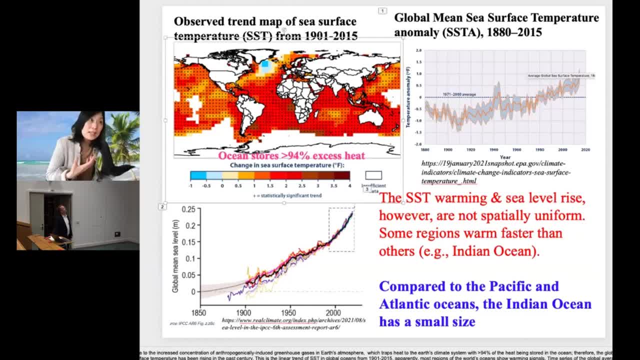 ENSO- tropical Pacific Ocean circulation. the most dominant mode, we all know, is ENSO. Yes, So when we have a La Niña phase, that's a negative phase of ENSO. we have intensified The ensul, We have intensified the flow, very clear. 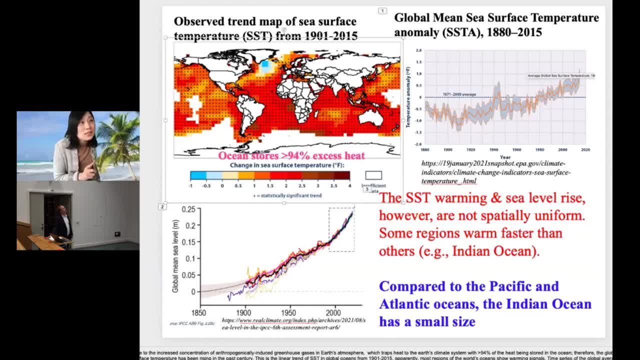 When we have a Niño phase, that's a warm phase of ENSO, and we have a reduced wave of ENSO. the correlations exceeding 0.8 is gold gases and gold to the Venus Almost allور. Inward students showed that problem as well. 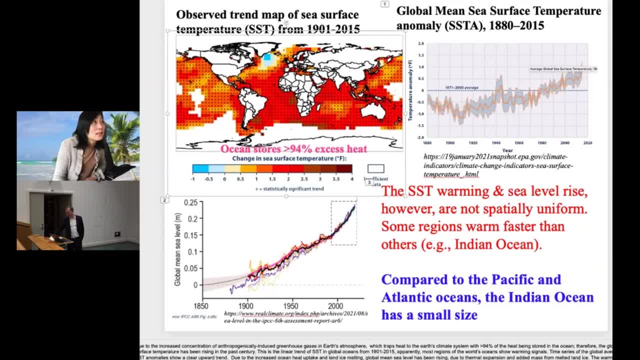 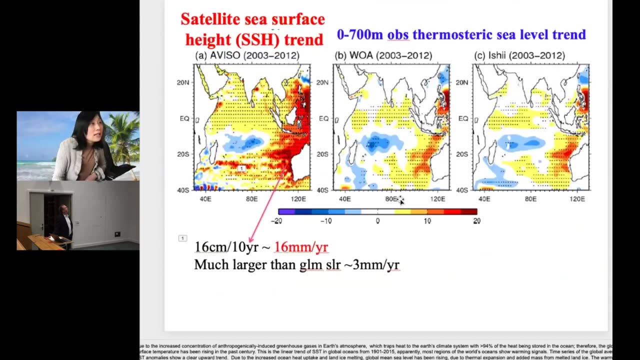 Earlier work, I think Susan Weevils and the sprinter also showed the high correlation between the indonesian through-flow and the ENSO And if we look at this, the hiatus period, and we show this, yeah, actually the intensified 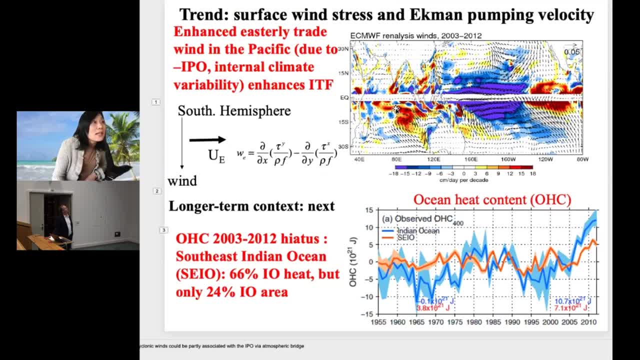 through-flow and the surface rent. that's a negative phase of inter-decadal pacific oscillation. The inter-decadal pacific oscillation on decadal time scale. if we do the filter of for Nino ENSO index like a year low-pass filter and calculate the IPO index and ENSO low-pass, 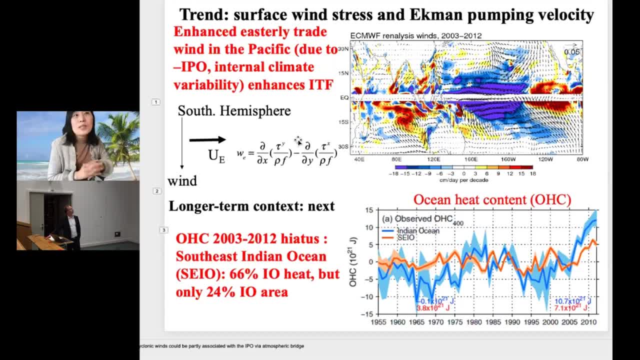 filtered index, the correlation is 0.89.. So therefore it's also under debate whether this decadal scale IPO mechanism, it's tied and linked to ENSO, decadal variability or the independent climate model. it's also under debate. 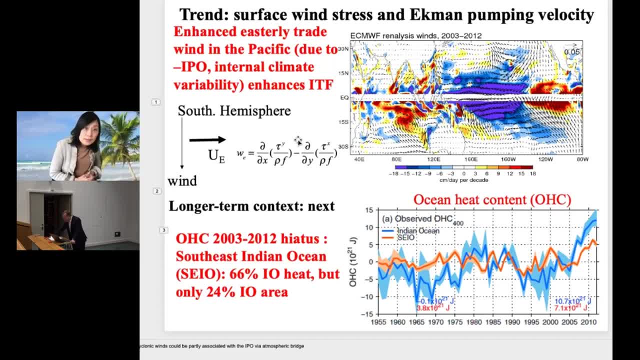 Okay, Thank you. I have here a comment more from Graham Quarterly. he writes: England and Wang or CLIM 2015, suggest that ENSO has effect on ITF lagging by eight to nine months, And he's wondering if you would know some more references on this. 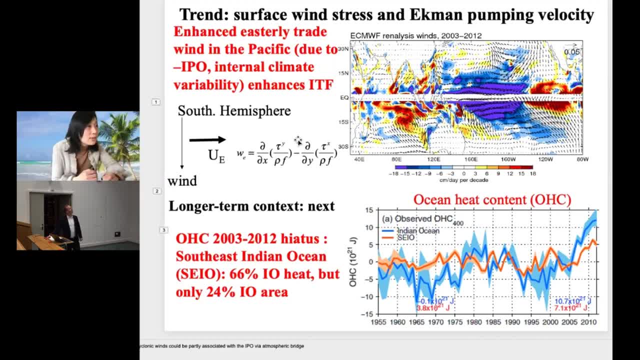 Yeah, afterwards if you send me an email. yes, I recently did do a lot, because I recently Arnold and I, Arnold did a lot. Yeah, There is a lag. you're right. Yeah, there is a lag. 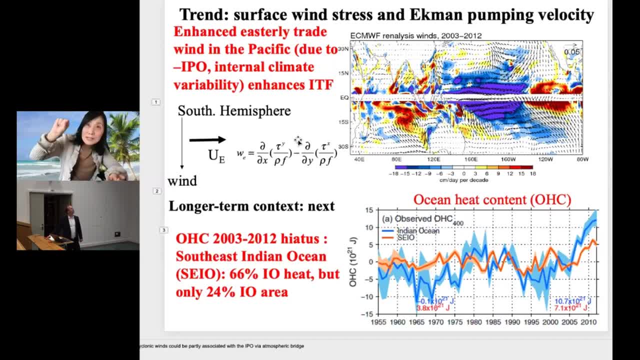 And especially if you look at the Makassar Strait. Makassar Strait is 80%, almost 80% of the Indonesian through flow that enters the Indian Ocean And Makassar Strait has a longer time series- I think 16 years right. 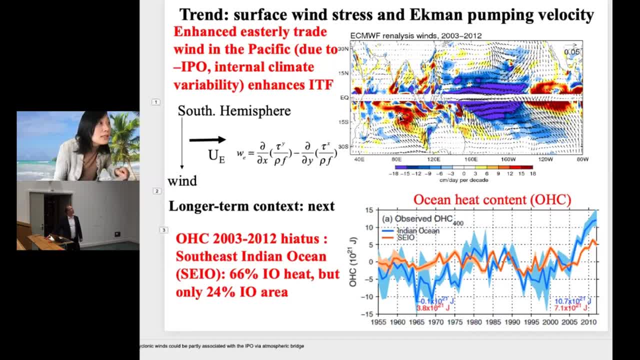 So instant, you know across here, like across here, they only have a few years, not continuous, But the Makassar Strait has the longest record. They also have a reconstructed. Maybe someone knows I'll find that reference and if you email me or let me know your email, 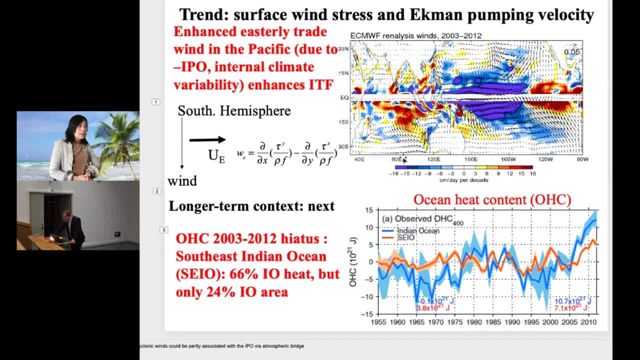 address. I'll find it Okay. Thank you very much. Thank you Great. And then there was a question from Annie and she says: what is the exact mechanism linking GHG and enhanced atmospheric circulation, hence stronger earth-easterliness in the IO? 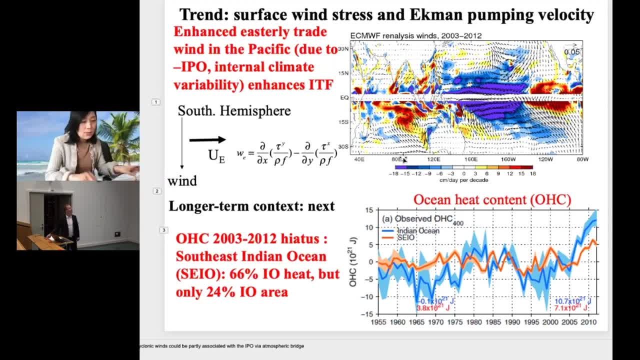 Yeah, Yeah, Okay. So greenhouse gas, Okay, Oh yeah. Yeah, That's a good question. Let's look at it. Did I Let me? I might have an additional slide. I'll put it here. No, I didn't. 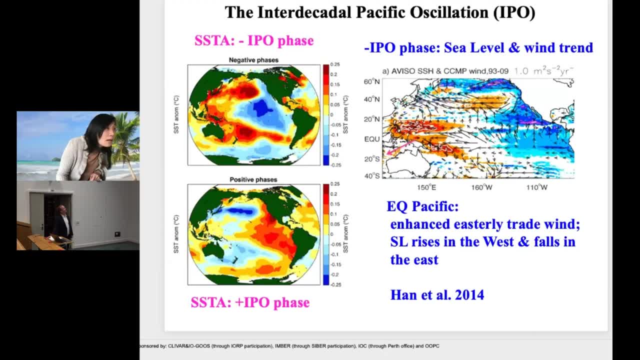 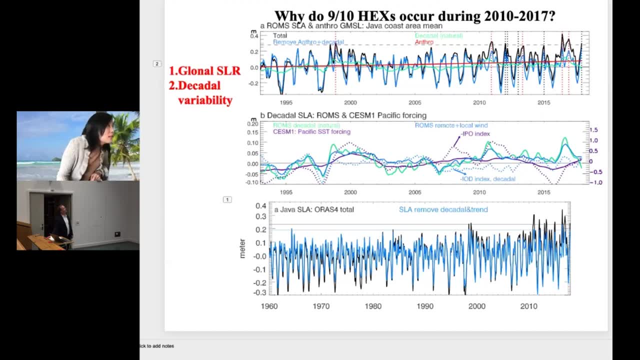 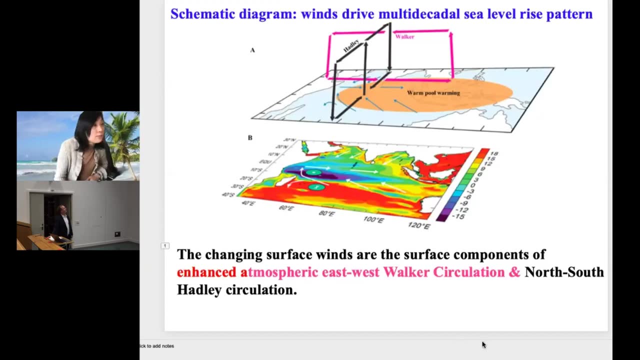 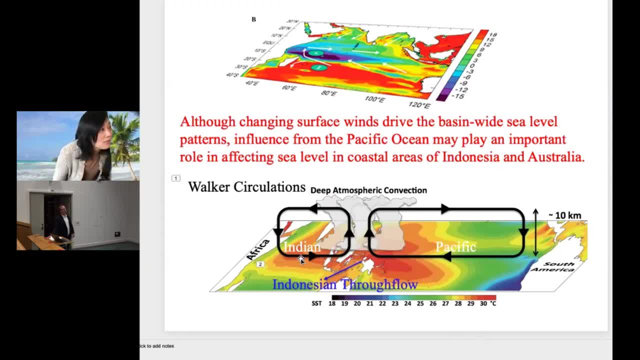 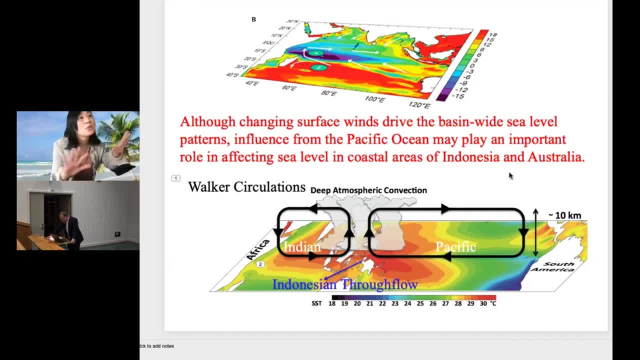 Okay, Okay, Okay. we have uniform warming. To make things simple, we have uniform warming throughout this Indo-Pacific basin And here the mean sea surface temperature over the Indo-Pacific warm pool, that's the Eastern Indian Ocean, Western Pacific, you have mean SST exceeding 28 degrees and 29 degrees C. 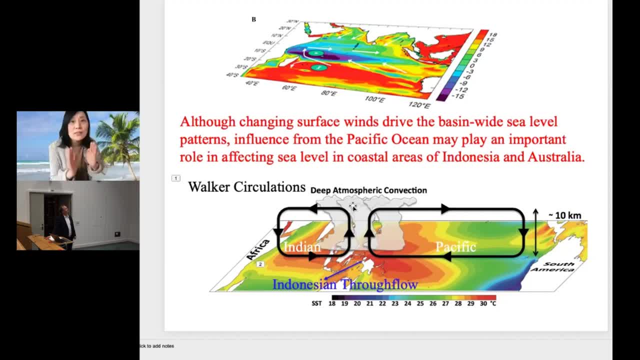 Atom spur convection, as I showed here, is very sensitive to the mean SST and the surface: wind convergence, moisture convergence. So when the mean SST exceeds 27.5, some people say 27,, some people say 27.5,, some people say 28,. okay. So when you have this, when the sea surface 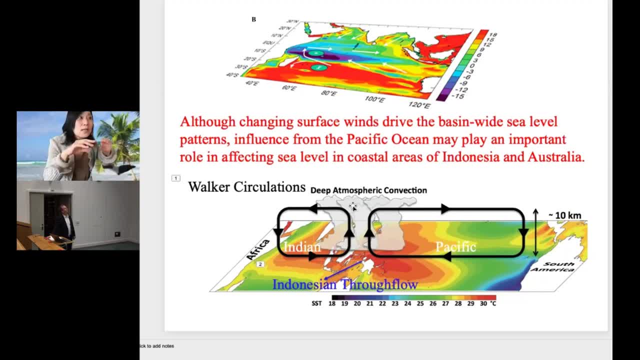 temperature exceeding a threshold, even a little bit change in the sea surface temperature, especially in the convergence zone, okay, and it has a dramatic increase in the convection, dramatic influence in the convection. basically it means that uniform warming added onto the mean SST pattern it wouldn't produce a 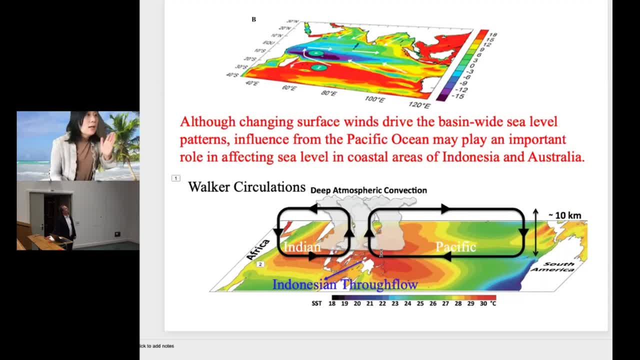 uniform convection or uniform wind. okay, In the high warm pool area you might intensify the convection and this intensified convection drives surface wind change. okay, That's possible, that's a possibility, okay. So if you have intensified convection, you have a. 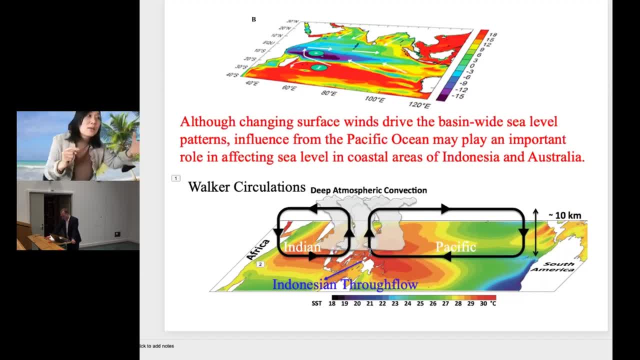 intensified the market circulation, so you have intensified west wind. Okay, so then did I answer your question, Annie. Maybe Annie will write back later. Let me maybe in the meantime, tell you the next question. So this is Lei Wang and he asks: a cooling trend occurred in the tropical southeast Indian Ocean? 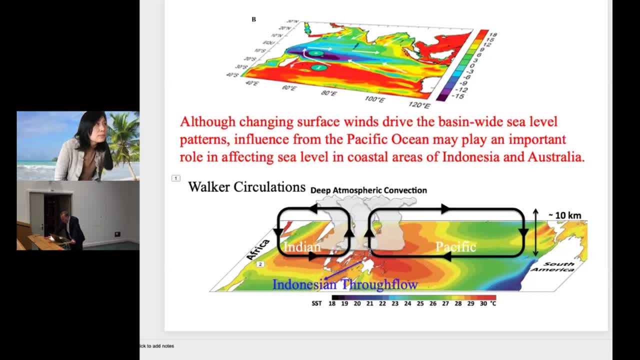 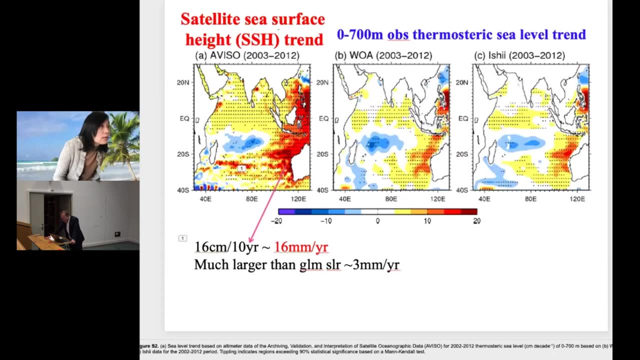 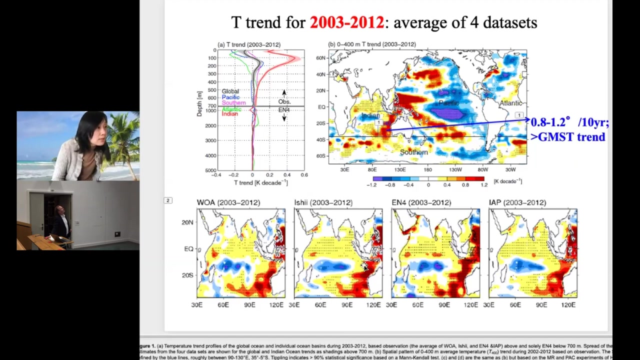 during 2003. to 2012.. Is this due to weakened SEC or local Ekman pumping? Which one is the cooling southeast Indian Ocean? Yes, and Annie writes that this was. thank you very much for the answer. It's just showing here. is that 2003,? that's the hiatus period talking about here, right? 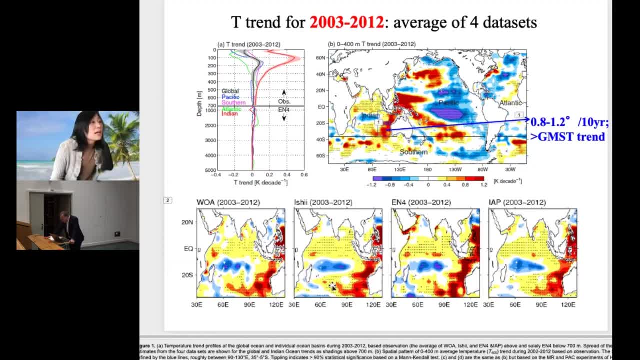 I guess. so, yes, Yeah, this one is, yeah, this one is actually consistent with our earlier work. yeah, And here: wind stress, wind stress pattern, wind stress curl pattern: this one It's, if you look at the wind. 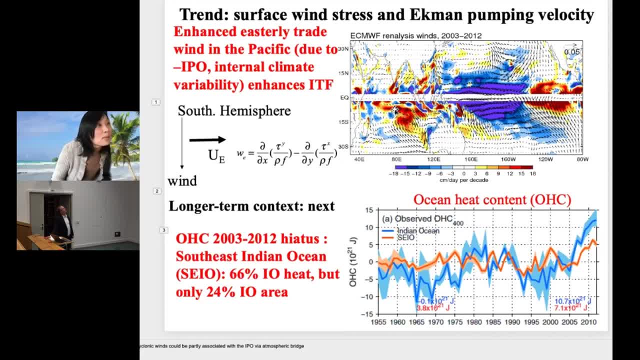 here, look at this red, this Ekman pumping velocity. that's this guy, this one WE. And when the WE Ekman pumping velocity is positive, we suck up the code of water to the surface, we cause surface divergence, cause upwards. So this is, this is actually consistent with our 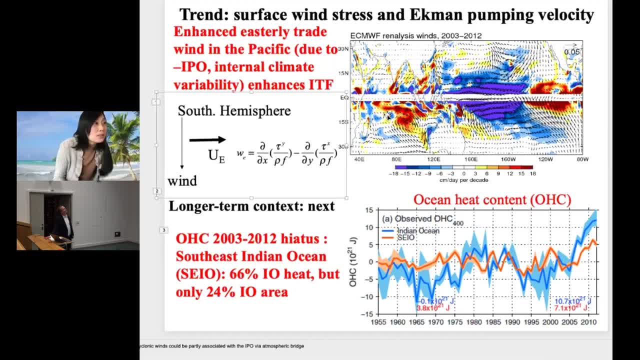 operating, So you would cause a cold temperature here. okay, because the operating And you may say, oh, it should be. you know central basin, We know this raspberry crop getting westward, So you accumulate this toward west So you may not see this, the wind pattern and this sea. 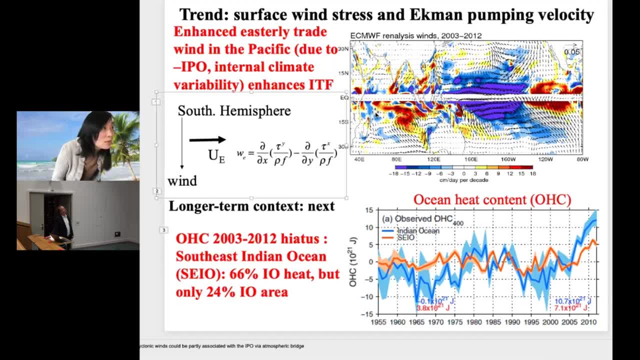 sea surface height or heat content pattern may be to the west a little bit compared to the surface wind WE Ekman pumping velocity. So this is: this is actually consistent with our operating So the wind WE Ekman pumping velocity pattern. Good question. 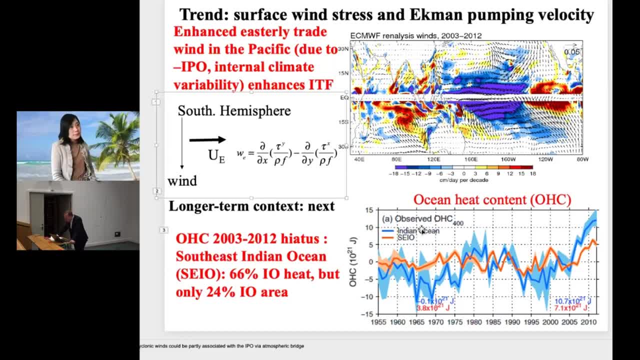 Thank you. Thank you very much. You have two more questions. So, Tony Songreich, excellent talk. Thank you very much. You mentioned two mechanisms, 코로나 and aстрonumerin, For the IO, IO- 산� Hertica. Do they enhance each other? 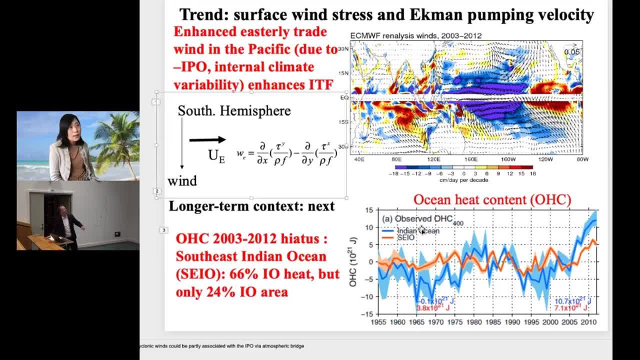 So is there a link? Do they enhance somehow More separate processes? Oh, okay, Assuming you, Tony, are the processes, but there are a few ones that we can use a little bit of mesh, Like you don't always have the increased to realize the mass power output here. So Oh, okay, As you told that, the resistance to a grounded H2, petri shimmer and H2 VIC, and you are increasing this wind wind accuracy. that can give us a point of curve, but it's easier to see briefly, So 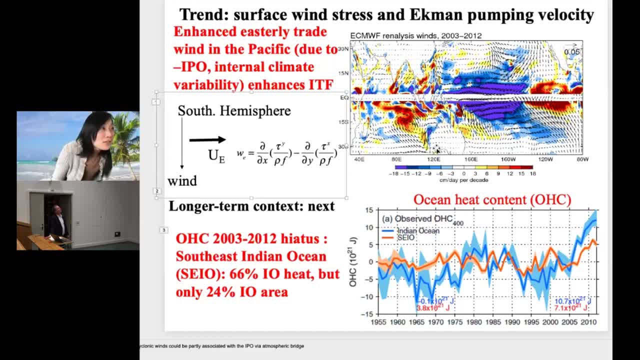 the intensified through flow is the source of this heat increase in the Indian Ocean, but where the water will store in the Indian Ocean, determined critically by the Indian Ocean window pattern. So this Indian Ocean, yeah, but regarding how, whether or not this surface window, 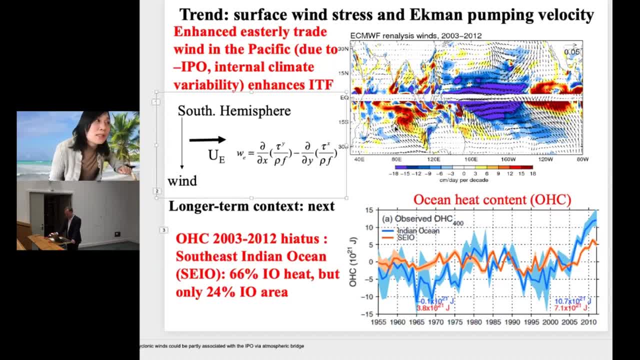 pattern also intensified through flow? we didn't do experiment to examine that, Thank you, And there is our last question by Ivan Orsoli: Is there a trend in the longitudinal Indian Ocean dipole associated with the intensified equatorial westerlies? 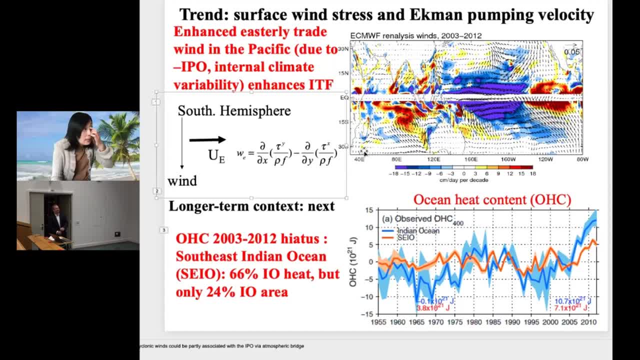 Westerlies, Oh yes, Oh. westerly wind, Oh okay. Yeah, there's recent work. I know you may be talking about this one. There are a debate regarding whether or not the equatorial Indian Ocean wax cell. 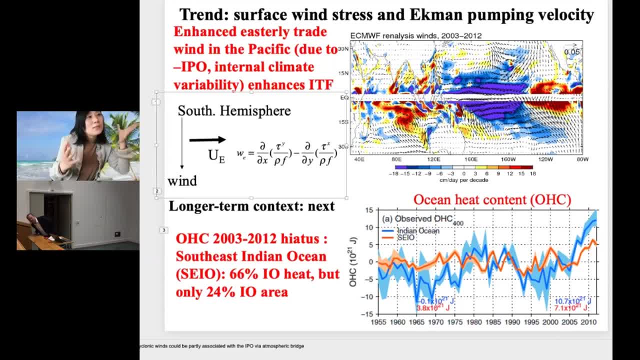 or even Pacific wax cell. we are seeing the Pacific wax cell right. it's weakening And also, you know, because of anthropogenic greenhouse gas forcing the Manila research and Manila research show. oh, we didn't see this in the observations or reanalysis data. 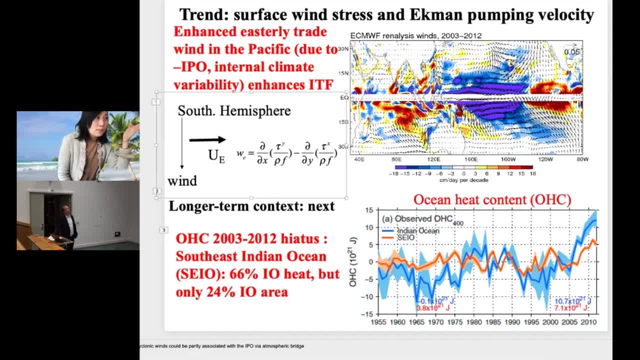 Okay, And the Indian Ocean. also there is debate. We talked about the intensified westerly wind, that's the intensified rock circulation pattern showing in different reanalysis products. but climate models shows that the Indian Ocean dipole in the warming climate will be. 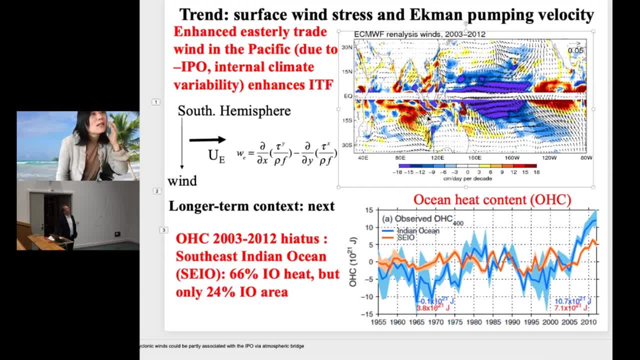 showing the intensified like positive dipole pattern, which means the eastern Indian Ocean: you have a colder SST. western Indian Ocean: you have warmer SST. If you think about this atmosphere ocean coupling, you would have intensified the easterly wind. But if you look at when the product it's very difficult to do this. 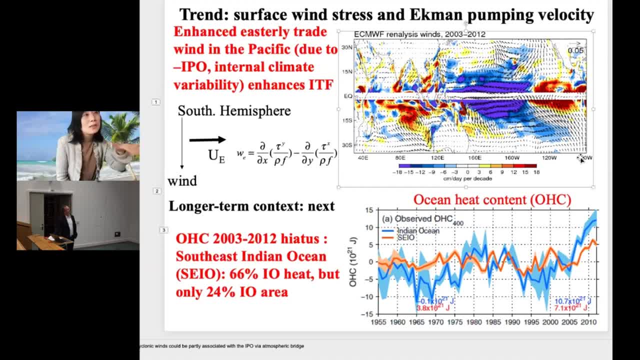 it's difficult to it is under debate, you know, when the product? we don't have a pretty long, reliable, long wind. So we do have this reanalysis window. I analyzed recently for different reanalysis when the product they converge in describing Indo-Pacific rock. 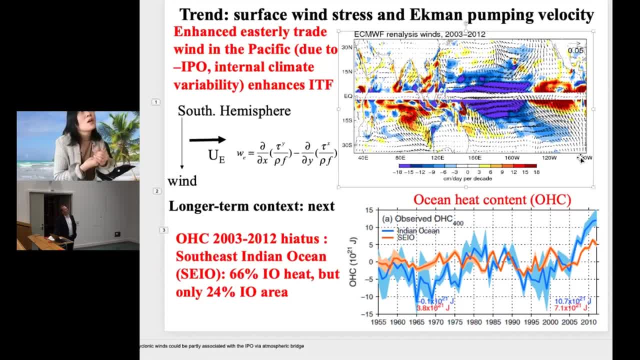 circulation. they converge, starting from 1967 also, or starting from early 1970s to the end of 1960s, Earlier than that. they're everywhere The reanalysis products. they do not converge even for describing this Indian and the Pacific surface branch of the rock circulation. 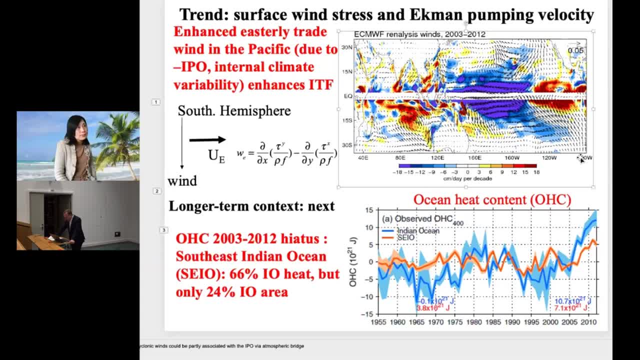 Thank you. Maybe also a last question from my side. Now. we just had the climate conference, of course, in Glasgow, with the goal of reducing the global warming to maybe 1.5 degree. Did you do any calculation what such an increase would mean for Indonesia, for example?